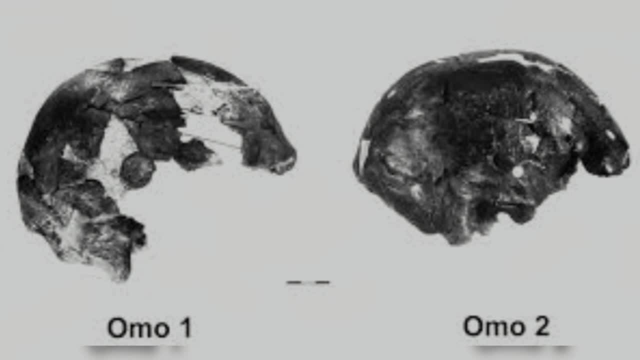 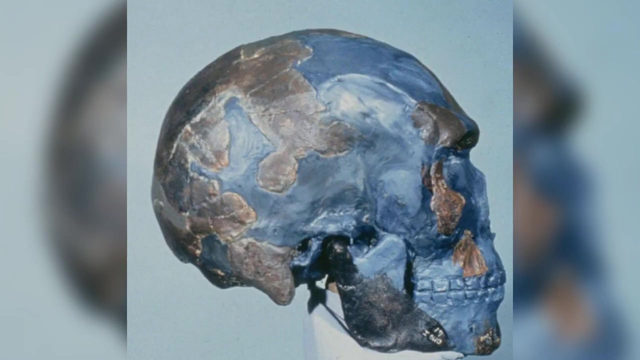 humans at that time. The Omo remains consist of two main specimens, Omo I and Omo II, with Omo I providing the most conclusive evidence of early Homo sapiens anatomy due to its more complete skull and postcranial bones. The features of the Omo I skull. 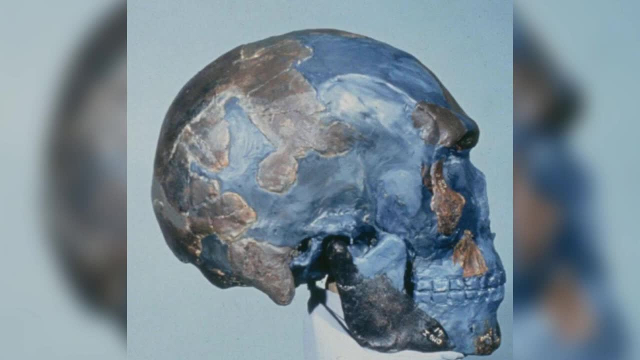 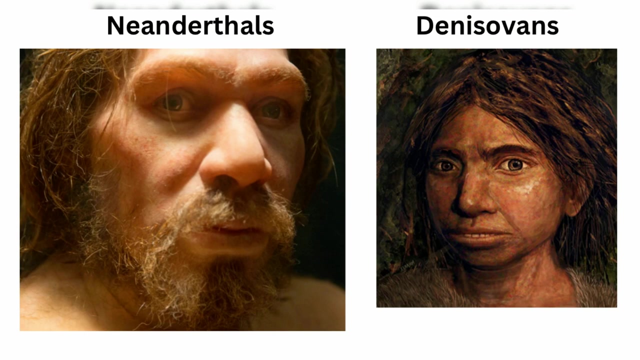 including a high forehead, rounded skull shape and reduced brow ridges, align closely with those of modern humans, distinguishing it from older hominin species. The age of the Omo fossils suggests that Homo sapiens coexisted with other hominin species, such as Neanderthals. 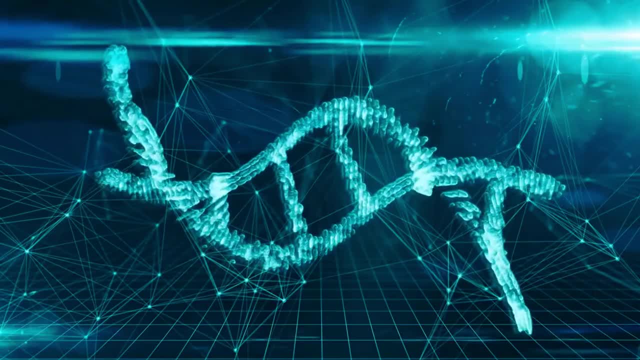 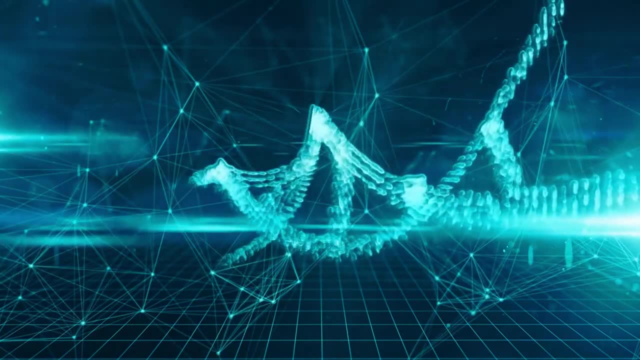 and Denisovans for tens of thousands of years. This coexistence has led to genetic intermixing, the traces of which are still present in the DNA of contemporary humans. outside Africa, The Omo Kibish formation continues to be an area of significant scientific interest. 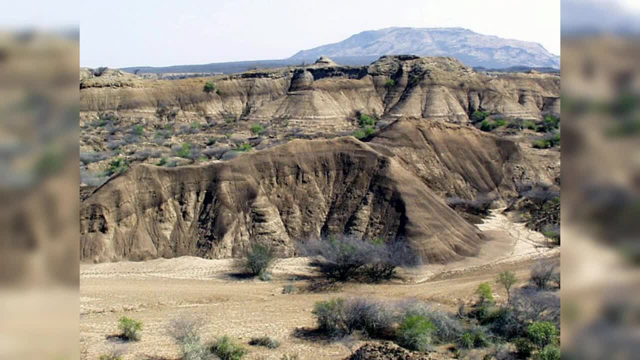 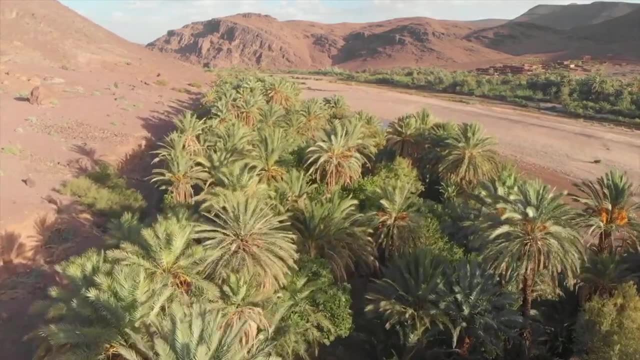 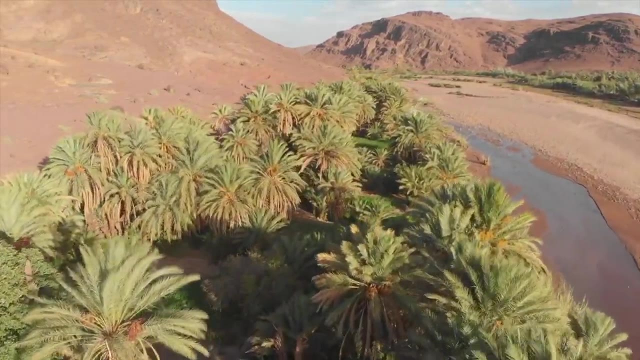 with ongoing research and excavations aimed at uncovering more about our ancient history. Now let's talk about a find in Morocco. The story of the Jebel Irhoud fossils begins in the 1960s, not with a search for the origins of humanity, but during mining operations in Jebel Irhoud. 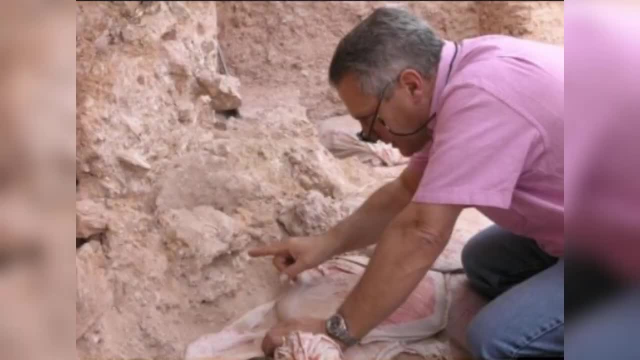 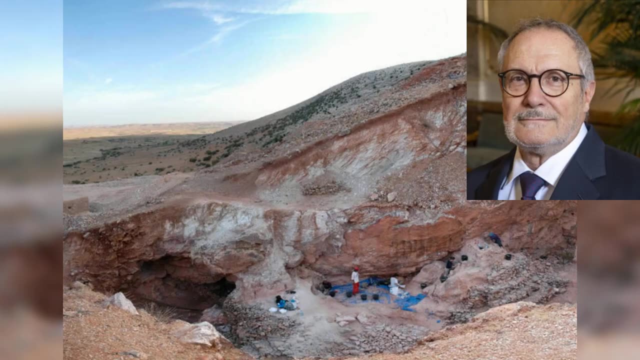 Morocco. The discovery of these fossils was somewhat serendipitous. Miners stumbled upon a few human skull fragments and tools, prompting further exploration. This site quickly caught the attention of paleoanthropologists, including a young French paleontologist, Jean-Jacques 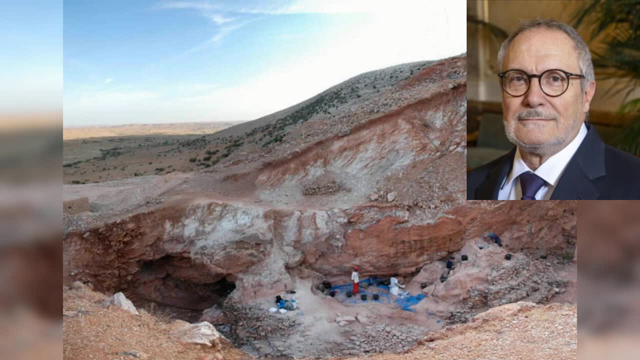 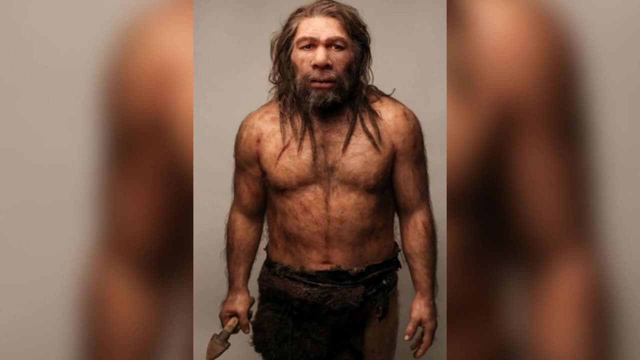 Oublun, who would later play a pivotal role in redefining the significance of these finds. Initially, the Jebel Irhoud fossils were thought to belong to Homo neanderthalensis and were dated to be around 40,000 years old, suggesting they were relatively recent Neanderthals. 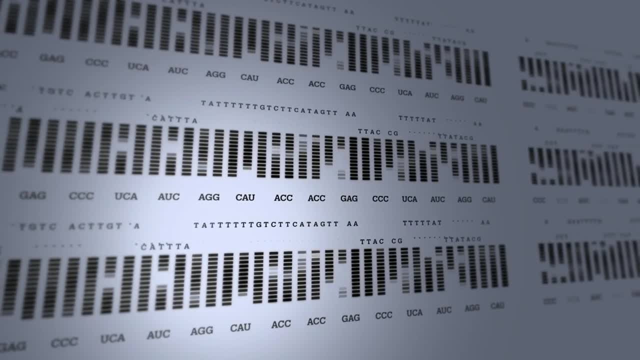 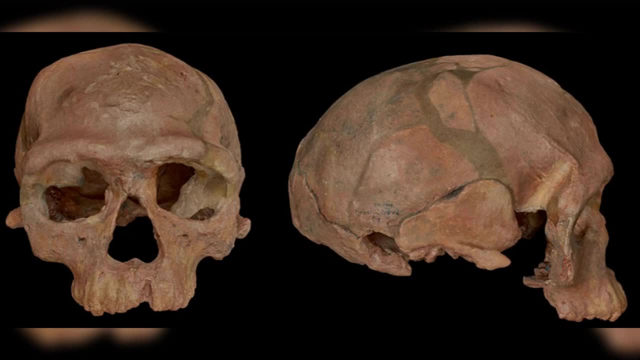 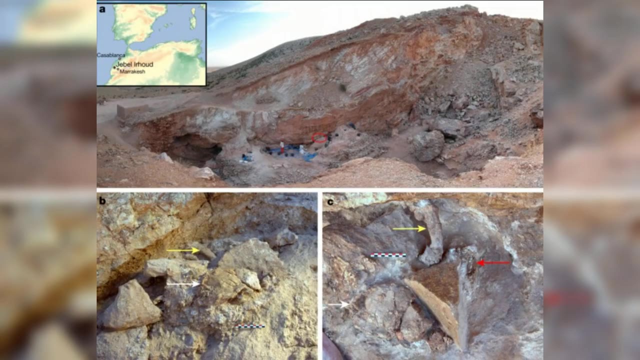 However, this initial classification and dating would not stand the test of time and technology. It was the advent of more refined dating techniques and a renewed interest in the site that would catapult Jebel Irhoud to the forefront of paleoanthropology In 2004,. Jean-Jacques Oublun. 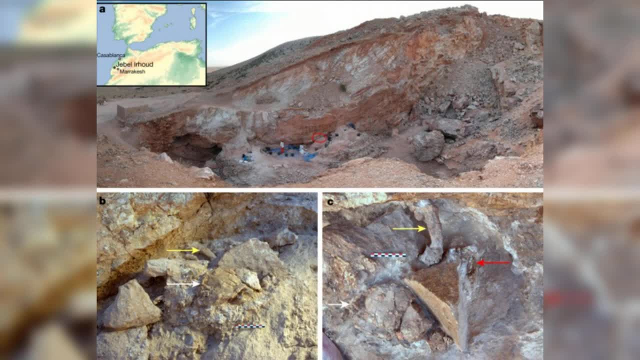 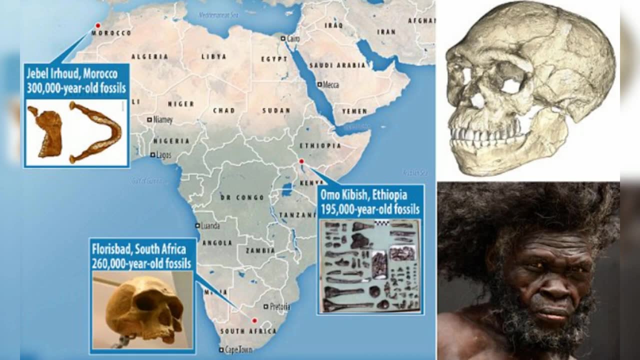 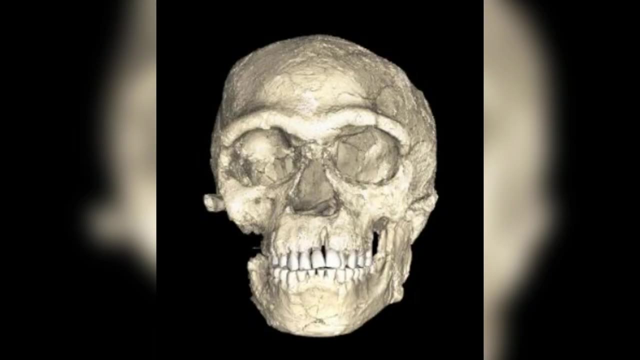 and his team returned to Jebel Irhoud with the intent of resolving the site's mysteries. Their efforts culminated in 2017 with the revelation that the Jebel Irhoud site was far more ancient than previously thought. Using thermoluminescence dating, a method that measures 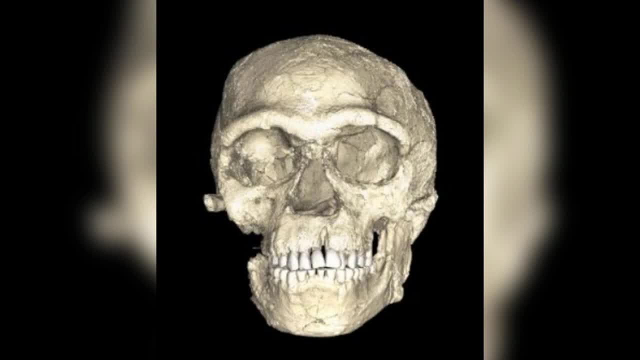 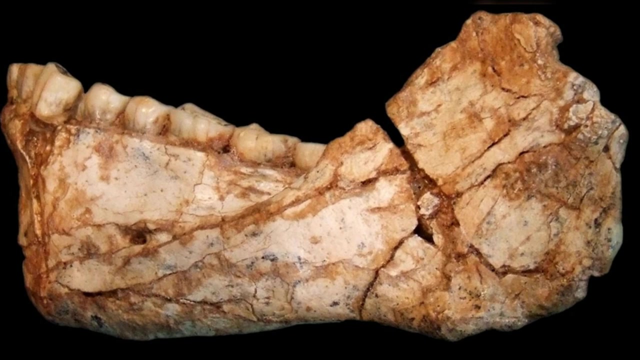 the light released when mineral grains are heated. the team determined that the flint tools associated with the fossils were approximately 300,000 years old. This dating, corroborated by other techniques, indicated that the human remains at the site were of the same age, making them the oldest known fossils of Homo sapiens. 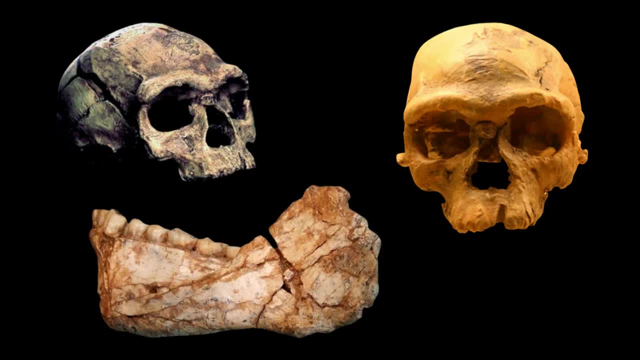 The Jebel Irhoud fossils include parts of several individuals, with the most famous specimens being a skull- Jebel Irhoud 1,- a jawbone and a partial cranium- Jebel Irhoud 10,- along with stone tools. 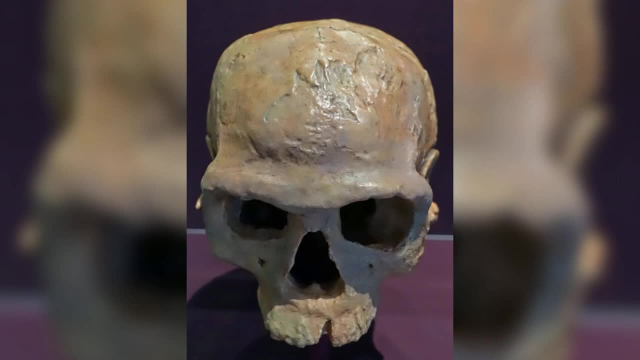 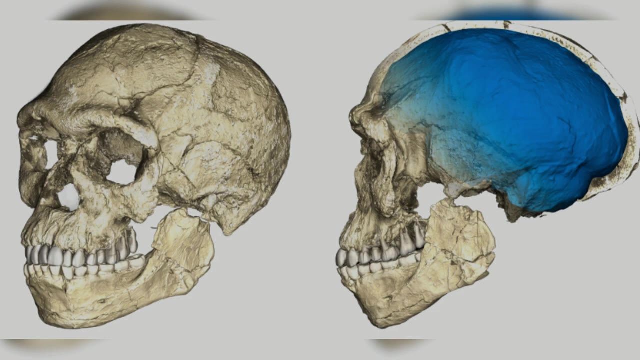 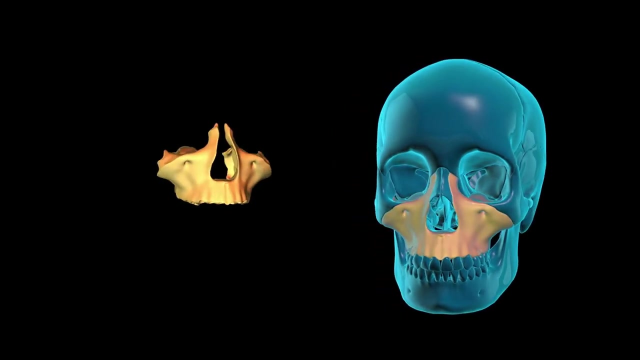 The morphology of these fossils, characterized by a mix of modern and primitive features, challenged prevailing models of human evolution. The skulls had a modern-looking face and teeth, but a more elongated brain case reminiscent of older human ancestors. This combination of features provided critical evidence that the facial 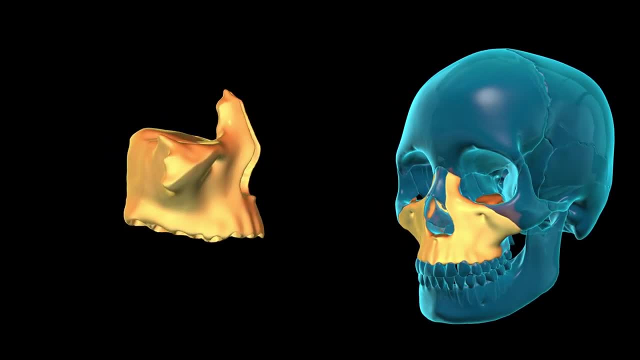 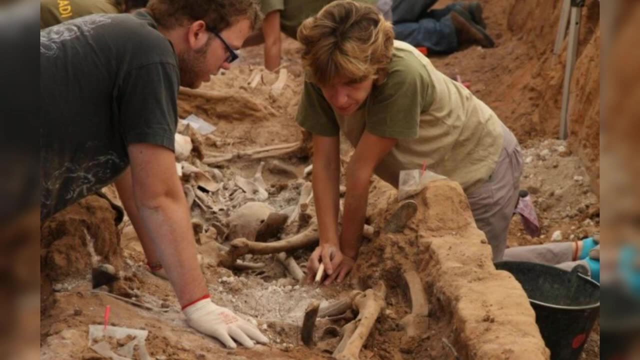 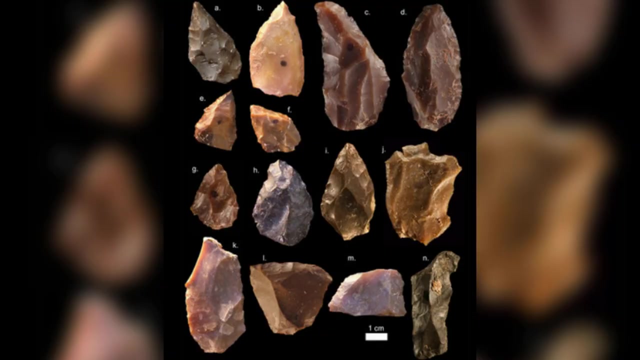 structure characteristic of modern humans appeared before the modern brain size and shape. The stone tools and animal bones found at the site provide insights into the lives of these early humans, indicating they were skilled hunters and toolmakers who utilized fire. The tools, part of the Middle Stone Age culture, represent a significant technological advancement. 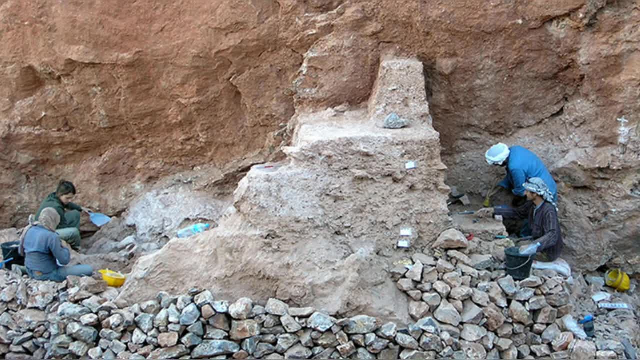 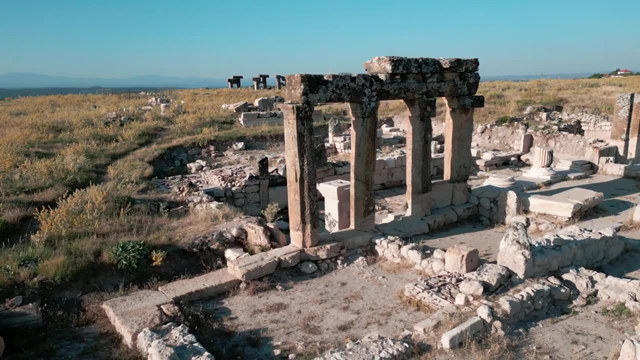 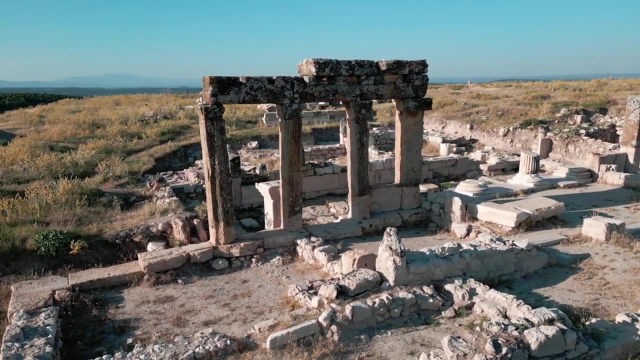 over older stone tool industries. The Jebel Irhoud site continues to be an area of active research, promising further insights into the dawn of our species. The story of its discovery and the revelations it has brought to light underscore the dynamic nature of paleoanthropology, where new finds 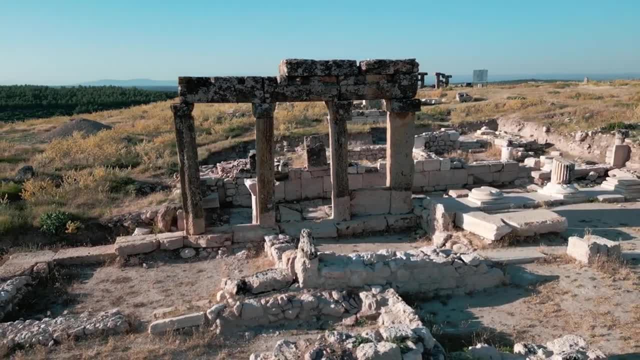 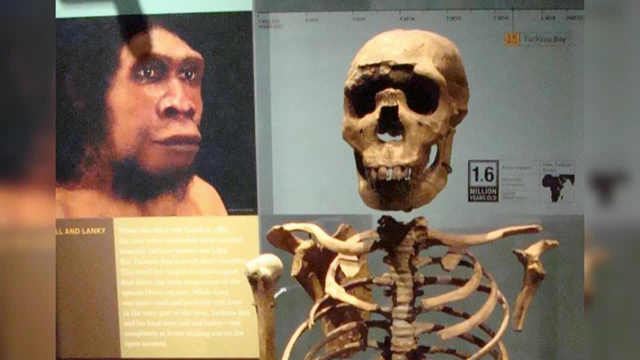 and technologies continually refine our understanding of where we come from. Let's learn about Turkana Boy now. The discovery of Turkana Boy, also known as Nariokotomboy, represents one of the most significant finds in the field of paleoanthropology. It was in the year 1984,. 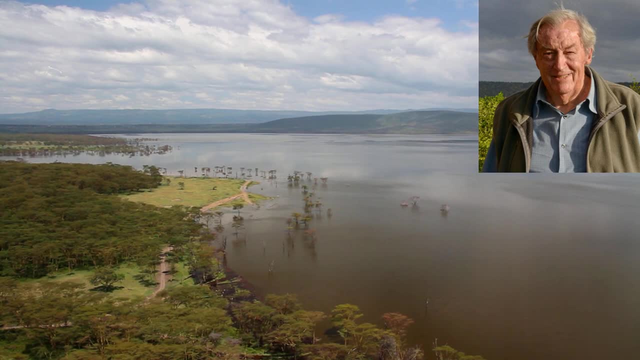 on the western shores of Lake Turkana in Kenya, that a team led by the renowned paleoanthropologist Richard Leakey, whom we have discussed already, made a groundbreaking discovery. Kamoya Kamu, a member of Leakey's team and one of the most successful fossil hunters in history. 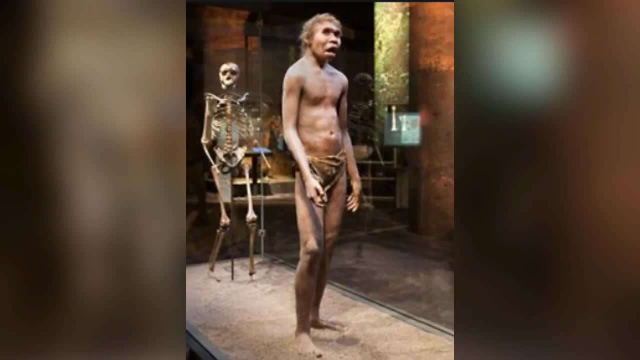 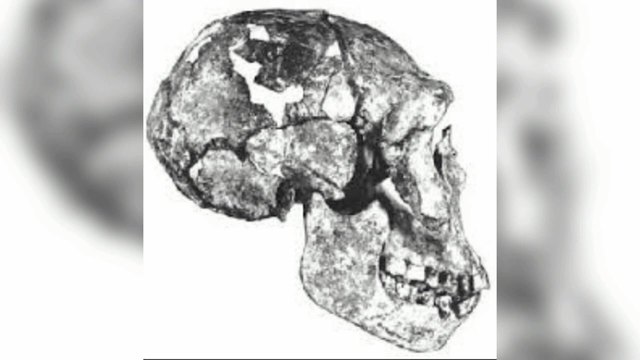 spotted a small shiny object on the ground. This object turned out to be a hominin tooth, which led to the unearthing of an almost complete skeleton of a young Homo erectus individual. The skeleton, catalogued as KNMWT 15000,, is estimated to be approximately 1.6 million. 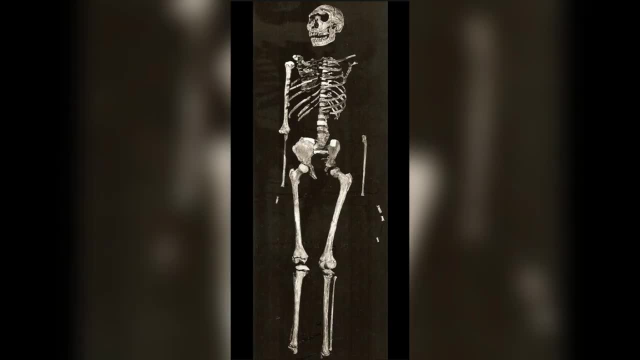 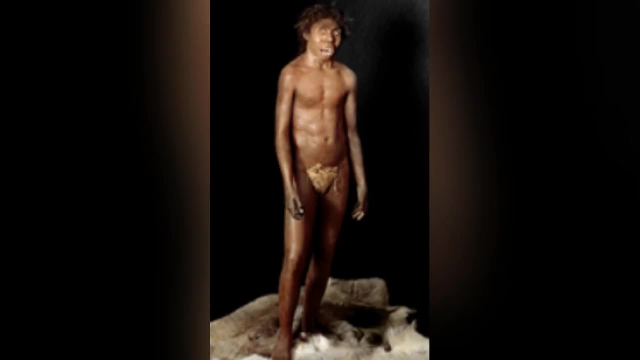 years old. It is the most complete early human skeleton ever found, with over 80% of the bones intact, excluding the hands and feet. Turkana Boy was a male and at the time of his death he was around 8 to 12 years old. 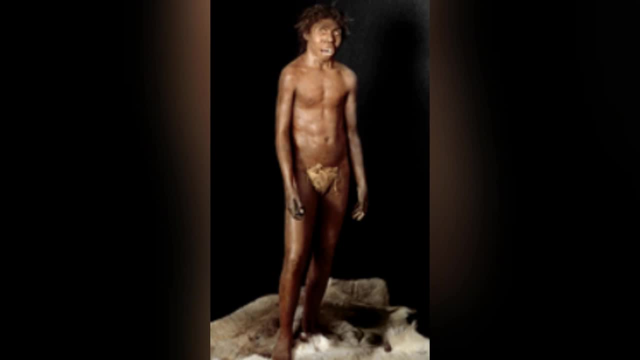 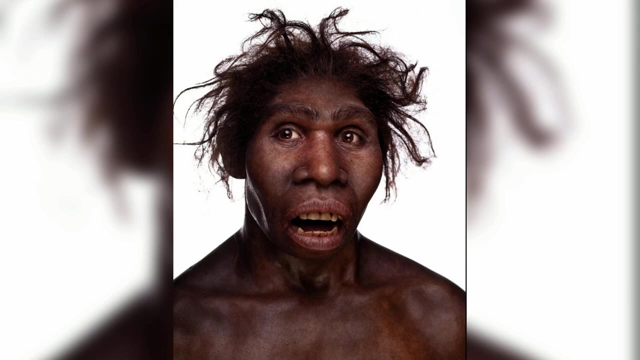 standing roughly 5 feet 3 inches tall and weighing about 106 pounds. Remarkably, analysis of his bones suggested that had he reached adulthood, he might have grown to over 6 feet tall. The importance of Turkana Boy's skeleton lies in the wealth of information it 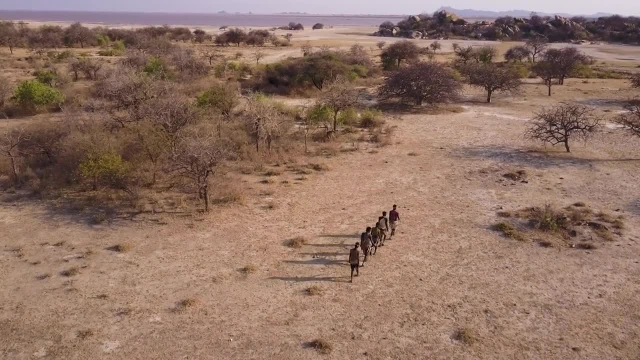 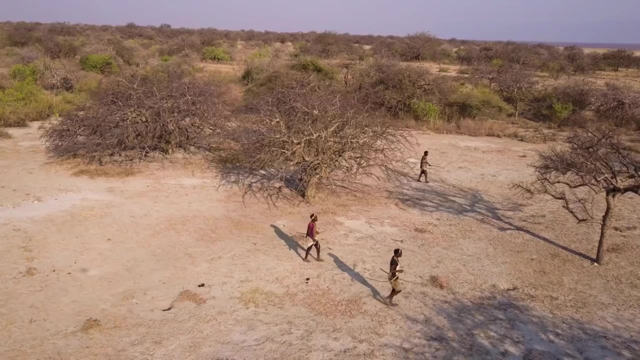 provides about the anatomy, growth patterns and health of the human body. Turkana Boy's skeleton, as well as the body of Turkana Boy, is a well-preserved skeleton which shows a mixture of primitive and modern features: The shape of his pelvis, the length of his legs. 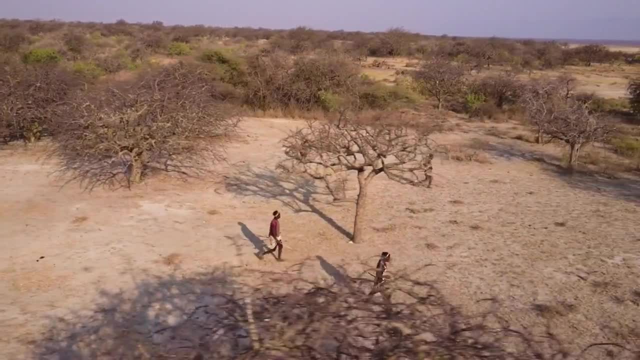 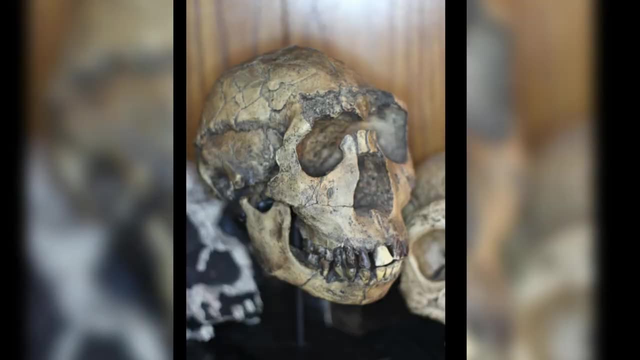 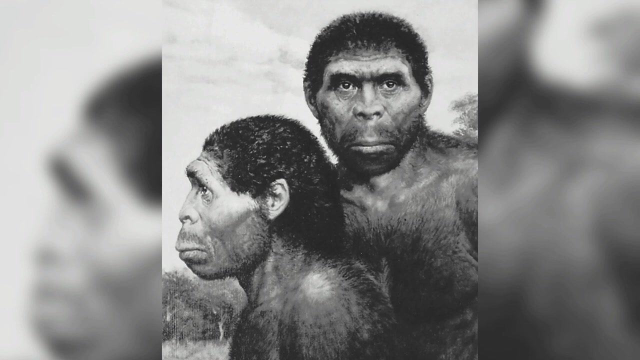 and the structure of his spine are all indicative of an individual fully adapted to bipedal upright walking, a hallmark of human evolution. Moreover, the size and shape of his brain case provide crucial insights into the evolution of the human brain: The discovery of Turkana Boy. 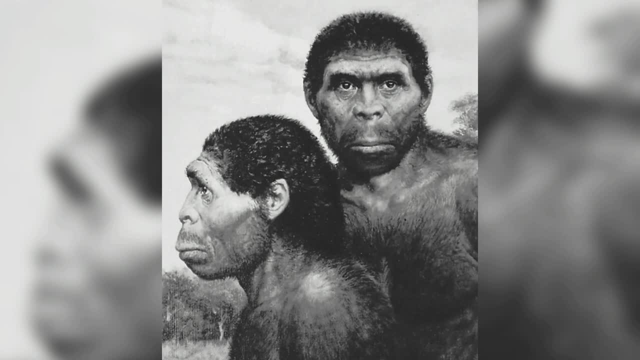 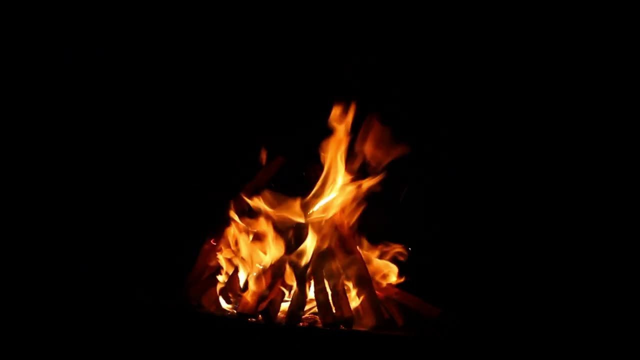 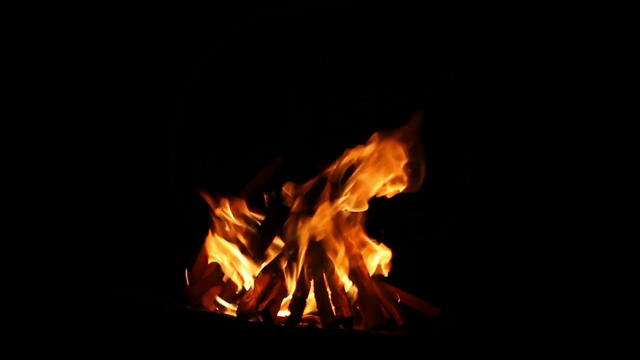 also contributed significantly to the evolution of the human brain, To our understanding of Homo erectus, a species that played a pivotal role in human evolution. This species is thought to be among the first to use complex tools, control fire and possibly even have a form of language: The almost complete skeleton of Turkana Boy. 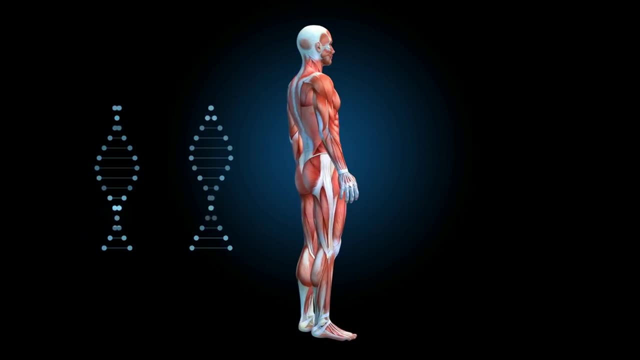 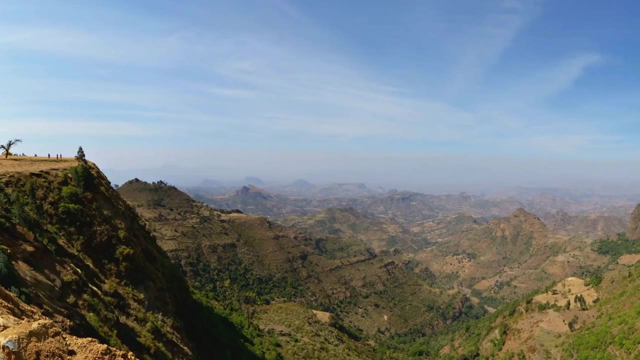 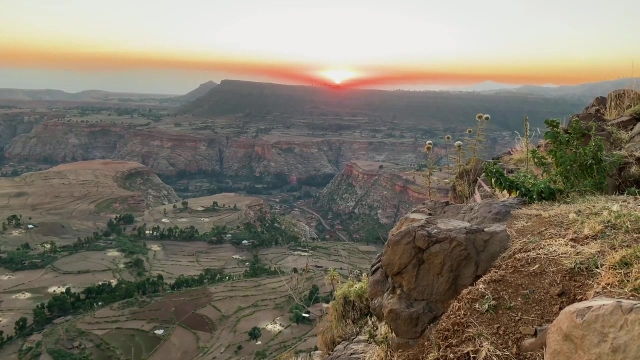 allows scientists to study the development and growth rates of early humans, offering clues about their maturation process compared to that of modern humans. Let's travel back to Ethiopia to know more about Ardi. The story of Ardi, short for Ardipithecus ramidus, began in the middle of. 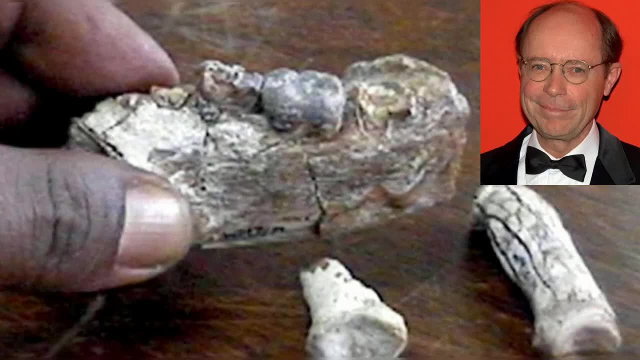 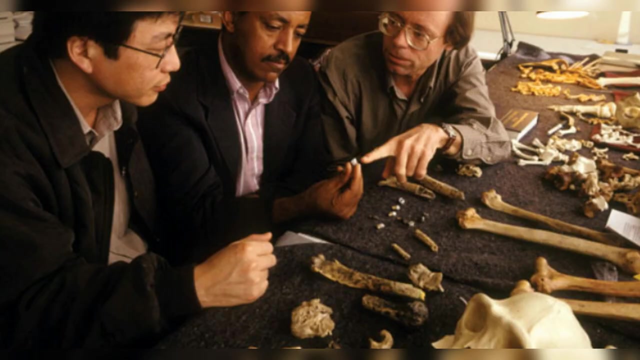 a desolate desert in the Afar region of Ethiopia In 1994,, a team led by Tim D White, an American paleoanthropologist, was meticulously surveying the area when they stumbled upon dental and bone fragments that appeared to be from an early hominin. These fragments were intriguing. 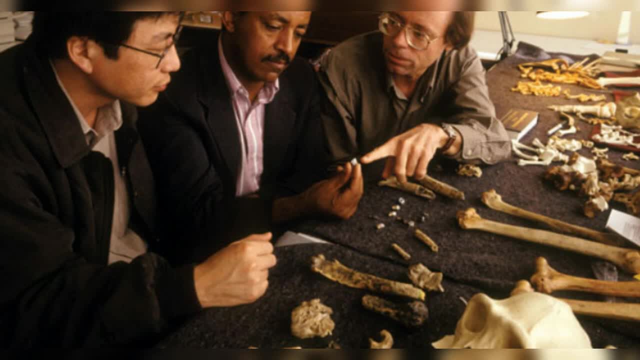 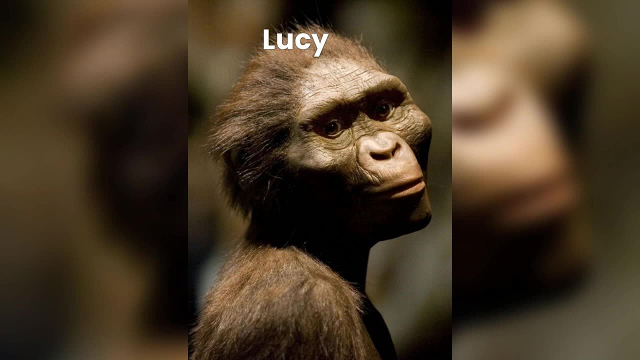 but it wasn't until the excavation efforts intensified over the following years that the discovery truly came to light. Ardi represented a major leap backward in time to 4.4 million years ago, significantly predating the famous Lucy Australopithecus afarensis by more than a million. 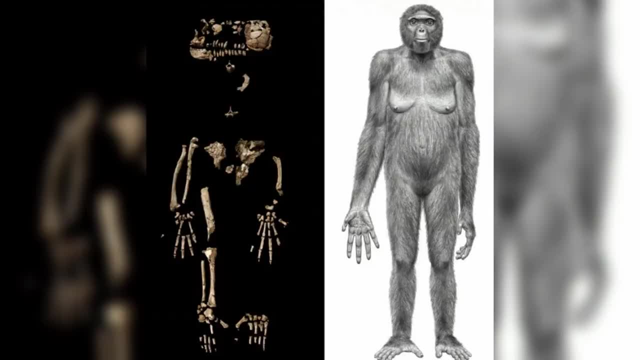 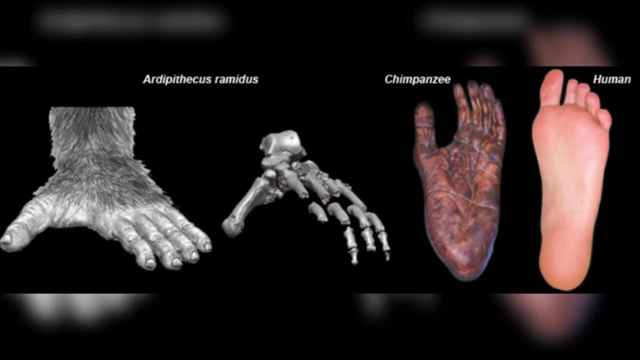 years. Unlike many other hominin fossils found in fragmented conditions, Ardi was remarkably complete, with more than 60% of her skeleton recovered. This degree of completeness is exceptionally rare in paleoanthropology. Ardi was the first to discover the origin of the human brain. Ardi was the first. 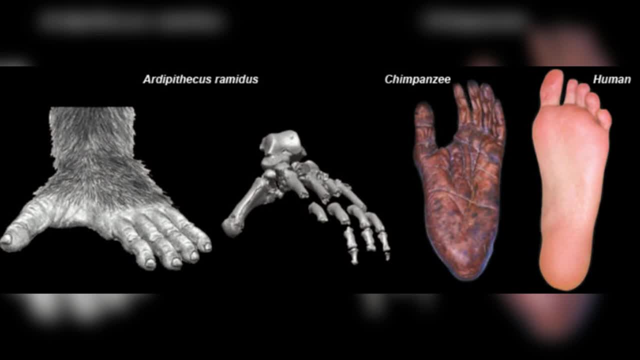 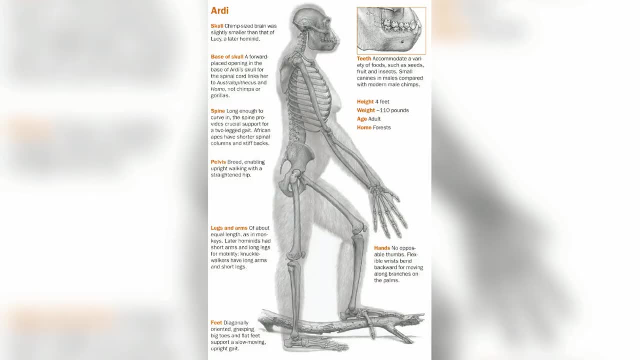 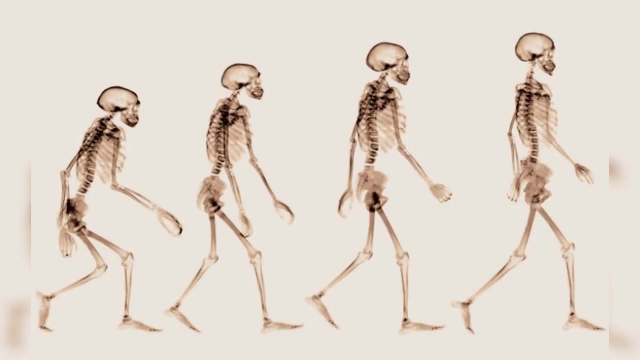 to learn morphology and provided an unprecedented opportunity to study the morphology and lifestyle millions of years ago. The publication of Ardi in 2009,, after 15 years of painstaking analysis, marked a pivotal moment in our understanding of human evolution. The findings challenged several 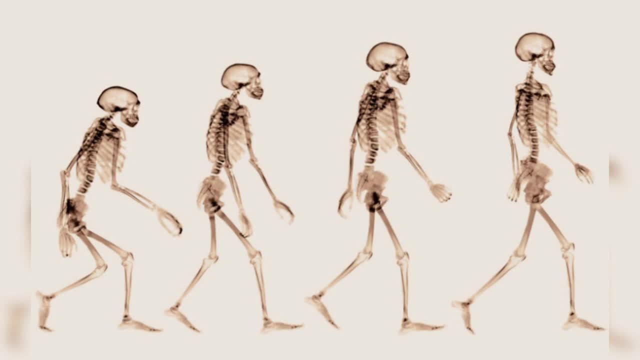 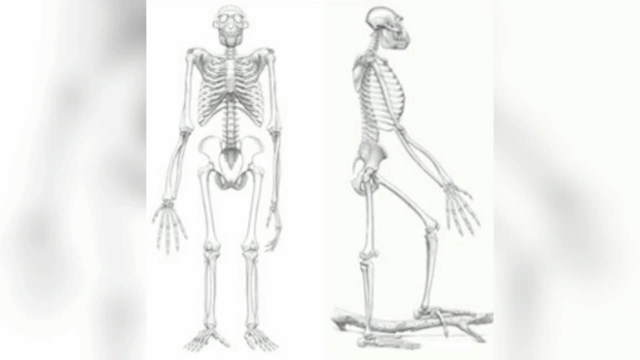 long-held beliefs about early hominins, particularly regarding bipedalism and social behavior. Ardi's physical structure suggested that she was capable of walking upright on two legs, yet her pelvis and feet indicated that she also spent time climbing in trees. This combination of 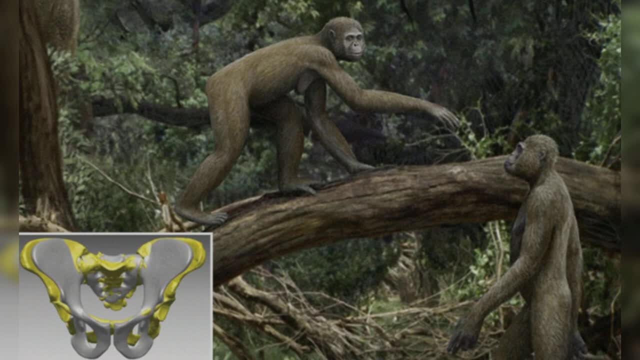 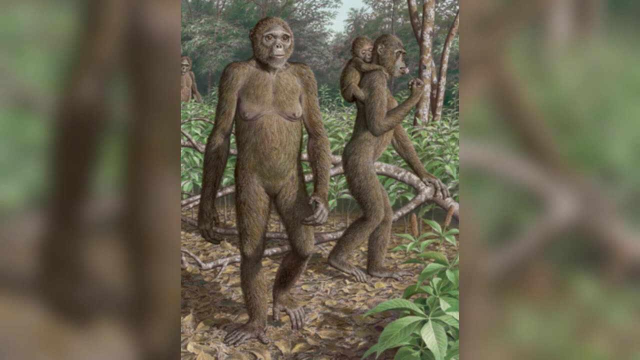 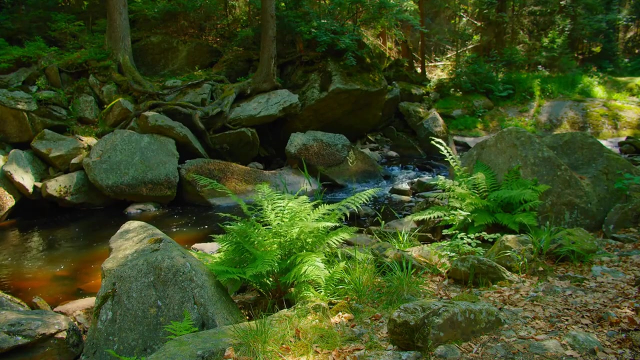 traits suggested a form of bipedalism that was quite distinct from that of later hominins like Lucy and modern humans. Additionally, Ardi's anatomy and environment provided clues about her lifestyle and social behavior. The region where she was found once a lush habitat with 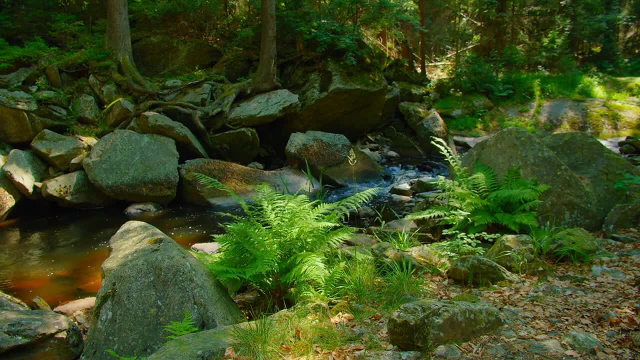 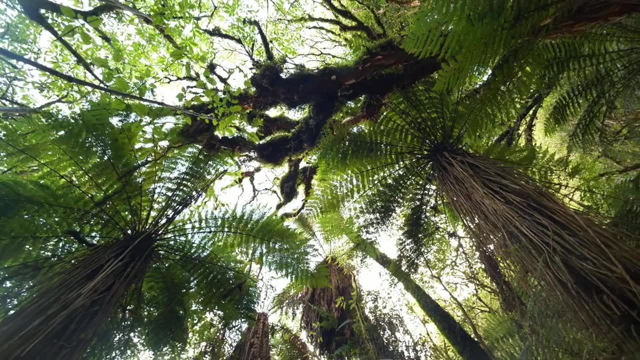 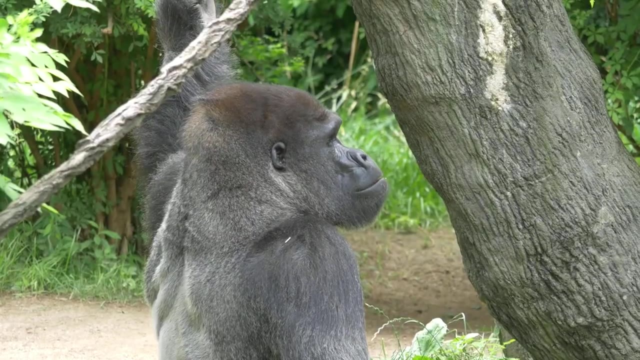 forests and lakes suggested that early hominins like Ardi lived in a more varied environment than the open savannas associated with later hominins. This environment would have influenced her diet, social interactions and locomotion in significant ways. Ardi's traits suggest that she may have 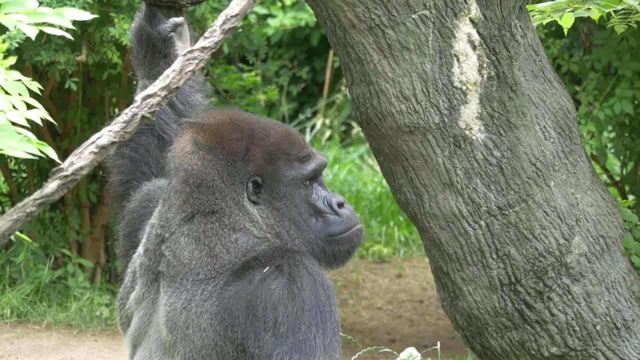 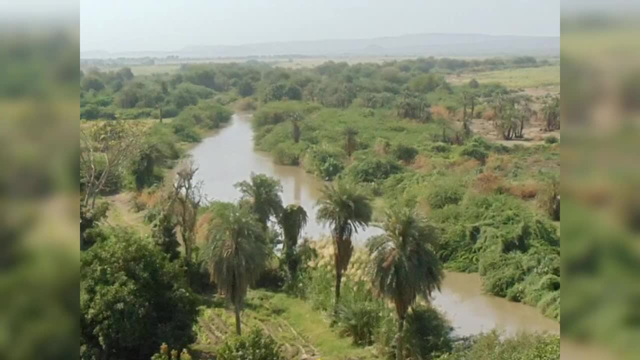 been less chimp-like than previously assumed, prompting a reassessment of how we interpret the behavior and morphology of chimpanzees and gorillas. Ardi's discovery near the Awash River in Ethiopia underscores the importance of the Afar region as a critical site for understanding. 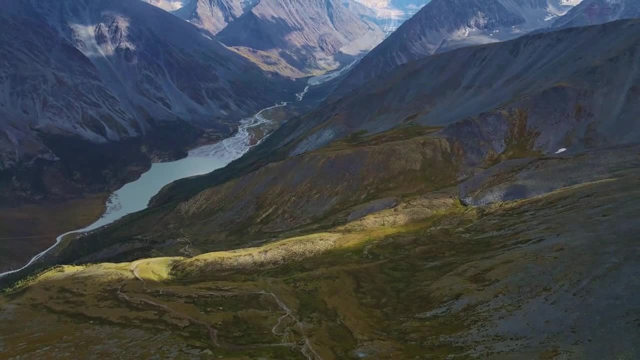 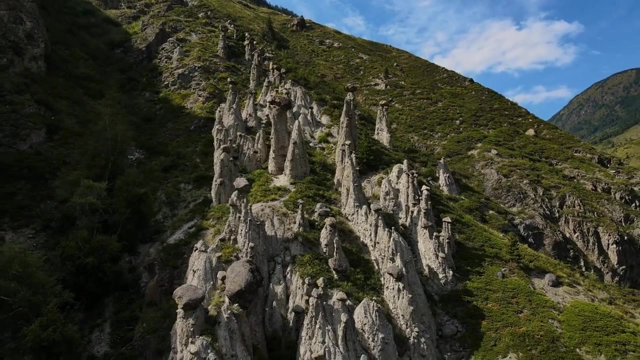 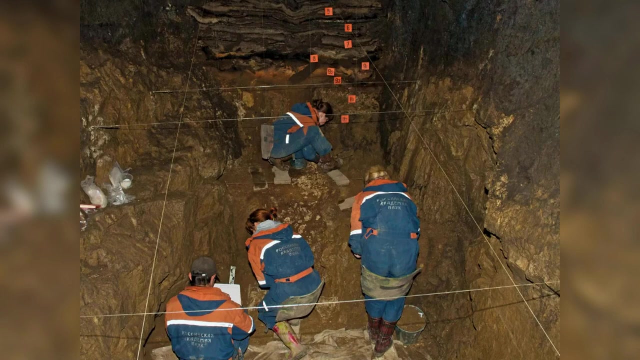 bipedalism. From Ethiopia, we now go to Siberia to know the enigmatic Denisovans. The story of the Denisovans, a mysterious group of archaic humans, begins in the depths of Siberia. The plot unfolds in 2010, within the chilly, remote confines of Denisova Cave. 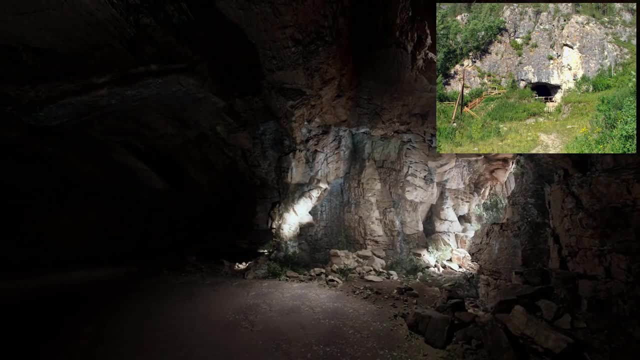 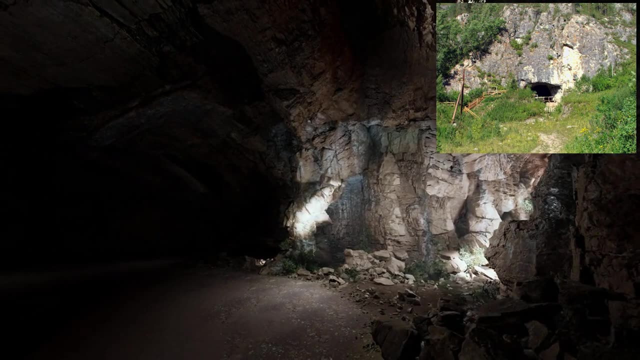 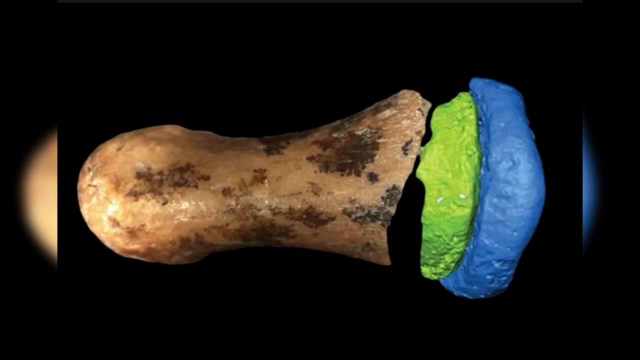 nestled in the Altai Mountains. This cave, already known to archaeologists for its rich array of hominin artifacts, was about to reveal a secret kept hidden for tens of thousands of years, The discovery began not with a complete skeleton, but with a single inconspicuous 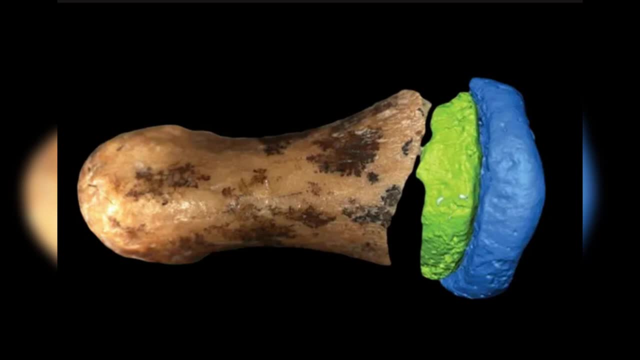 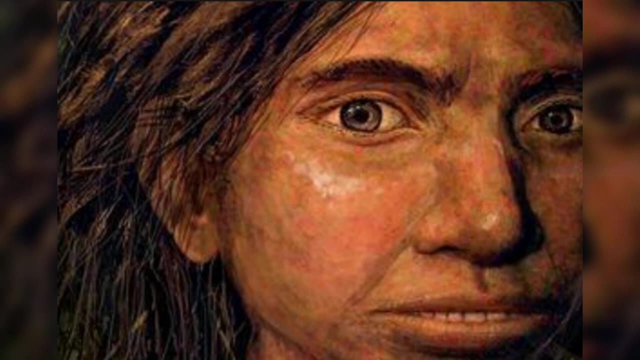 fragment of a pinky finger bone found in 2008.. This tiny fragment, belonging to a young Denisovan girl who lived approximately 41,000 years ago, would become the key to unlocking the existence of an entirely new group of ancient humans. Accompanying this find were two molars. 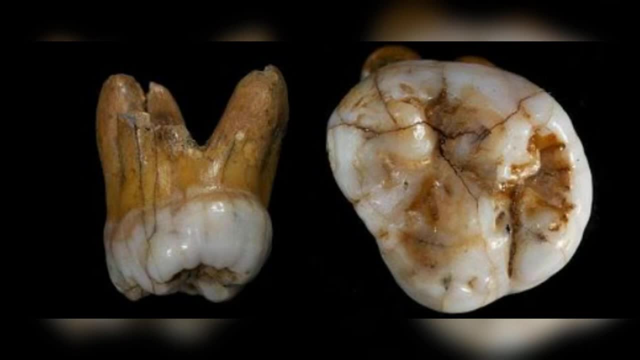 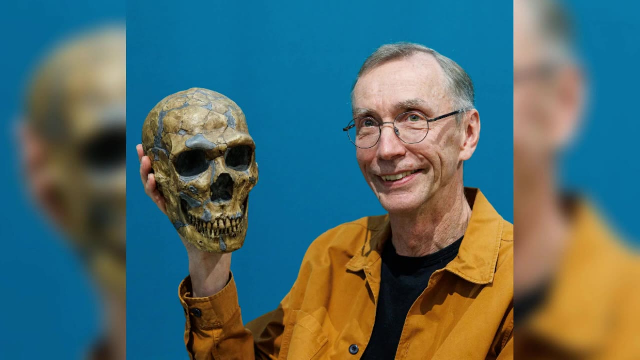 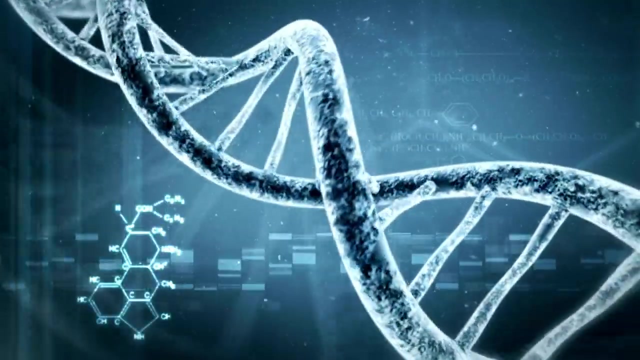 each robust and distinct enough to raise questions about their origin. In the yeah, the real breakthrough came when a team led by German paleogeneticist, Svante Paebo, performed genetic analysis on the finger bone. The DNA extracted from this fragment was remarkably well preserved, allowing Paebo and his team to sequence the Denisovan genome. 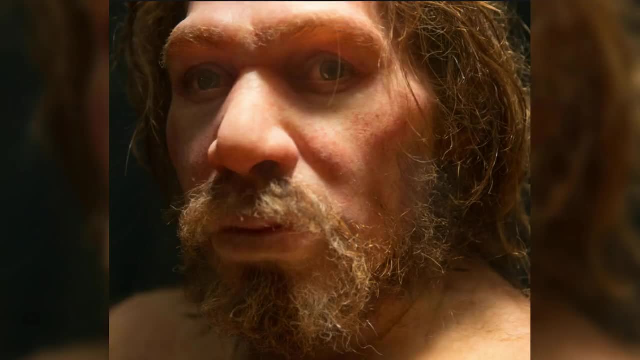 with astonishing accuracy. The results were staggering. The genetic material did not match that of Neanderthals or modern humans, indicating the existence of a previously unknown group of archaic humans. This was also the first time the DNA was found to be identified by the same group. 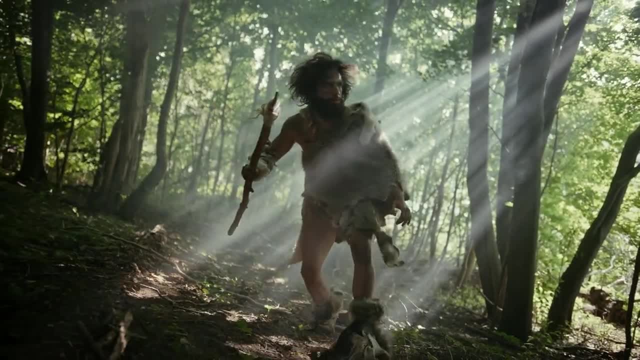 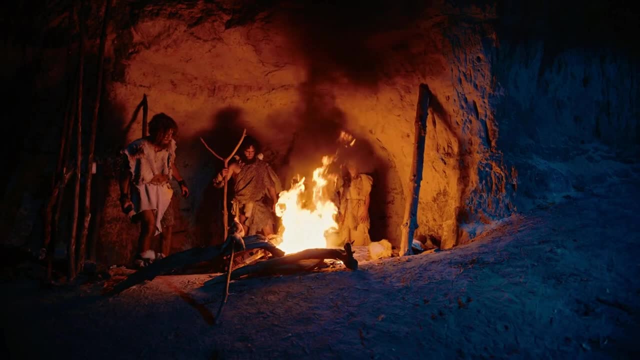 The Denisovans, as they were named after the cave in which they were discovered, revealed a complex web of interactions among ancient human groups. Genetic evidence showed that Denisovans interbred not only with Neanderthals, but also with the ancestors of modern humans. This interbreeding had a profound impact, particularly on populations in Asia and Oceania. For instance, modern Melanesians, Australians and other populations in the region carry up to 5% of Denisovan DNA, which has been linked to adaptations to high-altitude living among Tibetans and immune system responses. 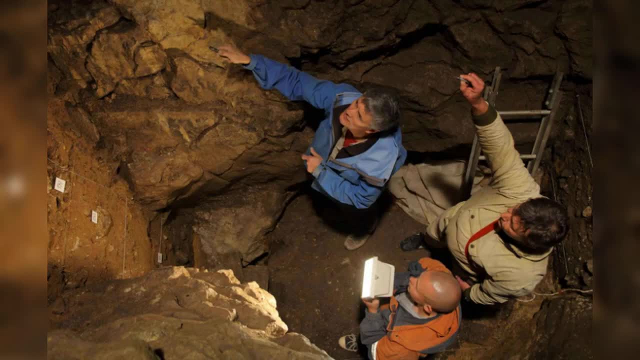 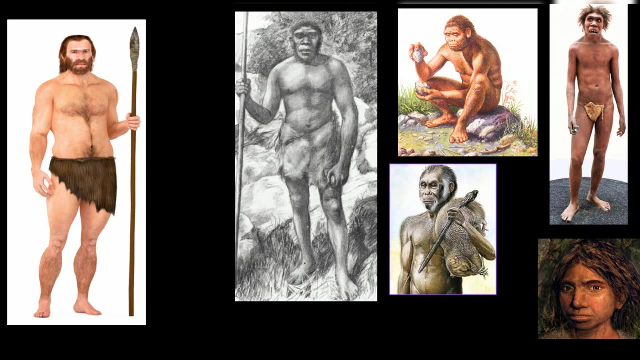 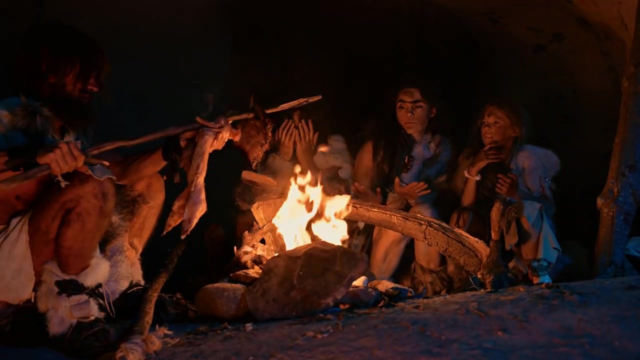 The implications of the Denisovan discovery are vast and varied. It highlighted the remarkable genetic diversity of ancient hominins and challenged the simplistic model of human evolution. The Denisovans, with their distinctive genetic traits passed on to modern humans, underscore the intertwined nature of human ancestry. 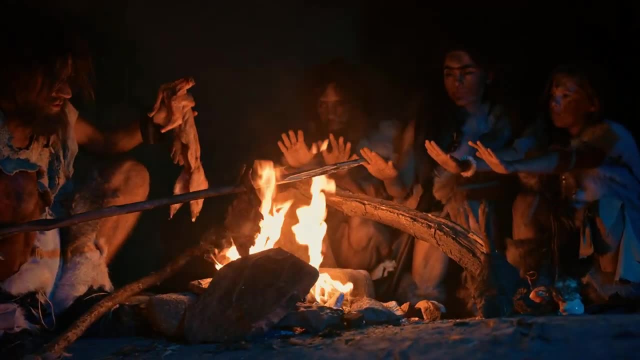 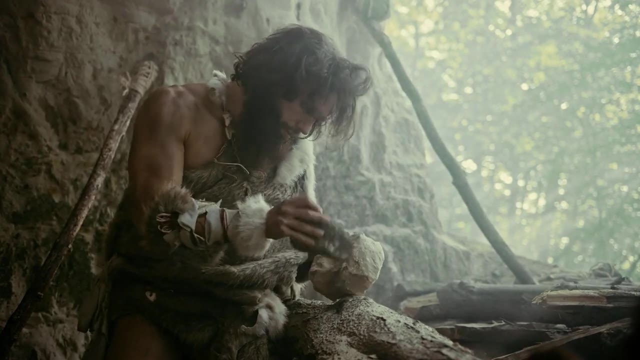 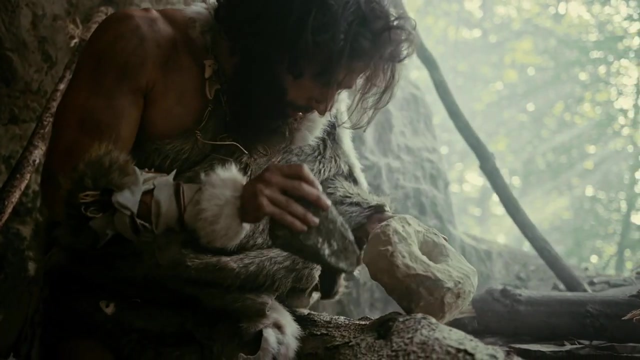 Demonstrating that our genetic tapestry is far more complex than previously believed. The identification of Denisovans fundamentally changed our understanding of human history, illustrating that the story of our past is not merely a linear progression from archaic forms to modernity, but a mosaic of interactions, adaptations and migrations. 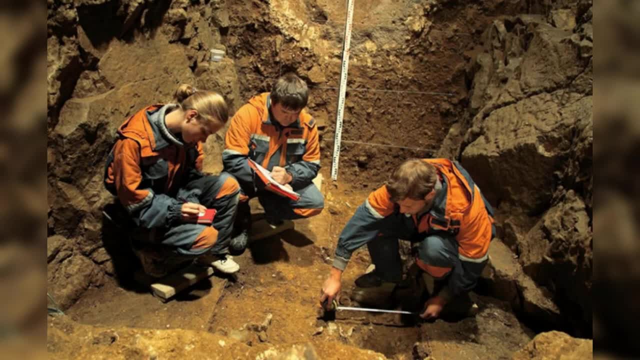 The ongoing research in Denisova Cave and the study of ancient DNA continue to reveal new chapters of this story, showing that our exploration of human origins is far from over. The tale of the Denisovans is a testament to the power of genetic science in archaeology. 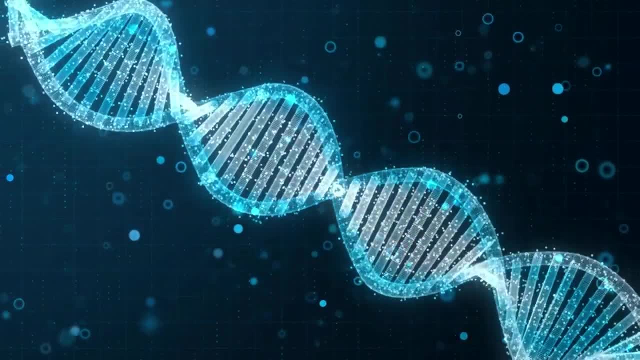 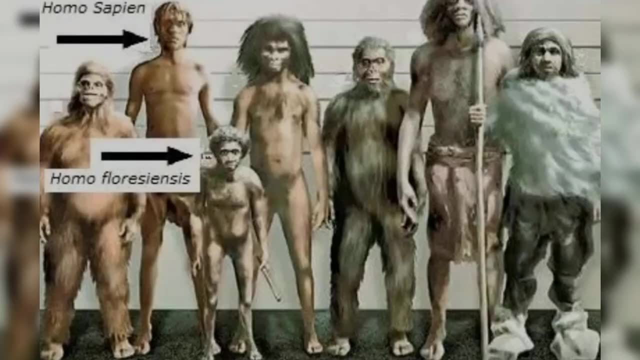 enabling us to uncover the secrets of those who walked the earth long before us. Let's us now go to Indonesia to learn more about a fascinating discovery. The discovery of Homo floresiensis and its diminutive stature reads like a chapter out of a fantasy novel. 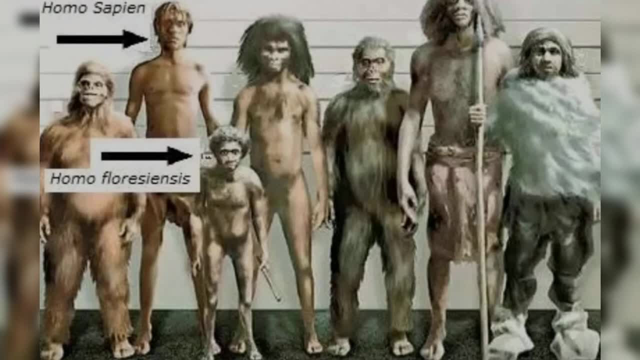 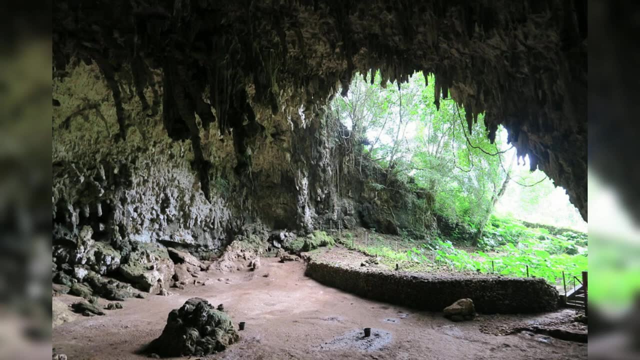 Yet it's a true story of scientific discovery that significantly altered our understanding of human evolution. In September 2003, in the Liyang Bua cave on the remote Indonesian island of Flores, a discovery was made that would send shockwaves through the paleoanthropological community. 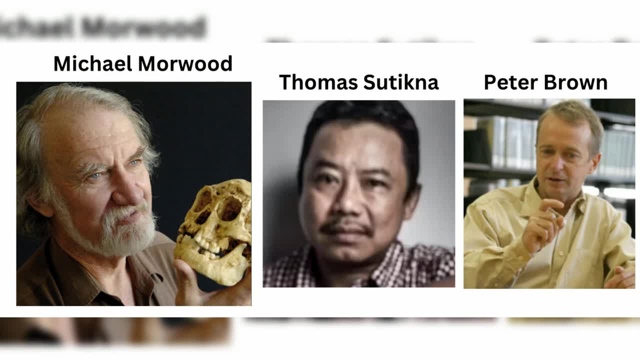 An excavation team led by Peter Brown, Michael Morwood and Thomas Sutikna unearthed the skeletal remains of a small-bodied hominin species that stood about 3.5 feet tall and had a brain roughly the size of a grapefruit. This find was astonishing. 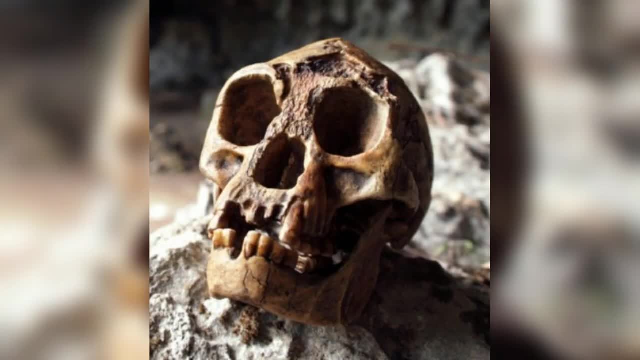 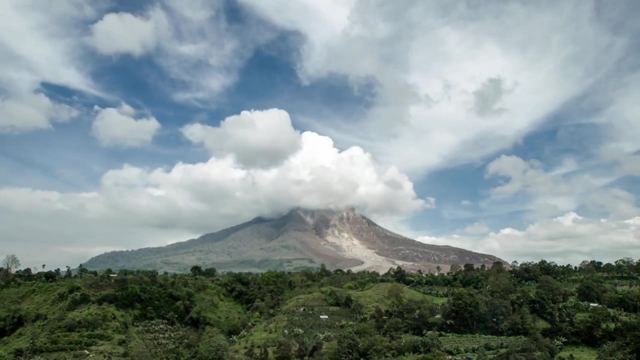 For several reasons. Firstly, the initial skeleton designated LB1, was dated to just 18,000 years ago, meaning this species coexisted with modern humans for a significant period. This timeline challenged the prevailing notion that Homo sapiens were the sole. 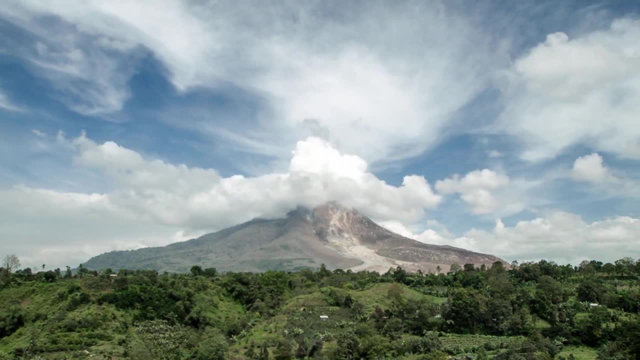 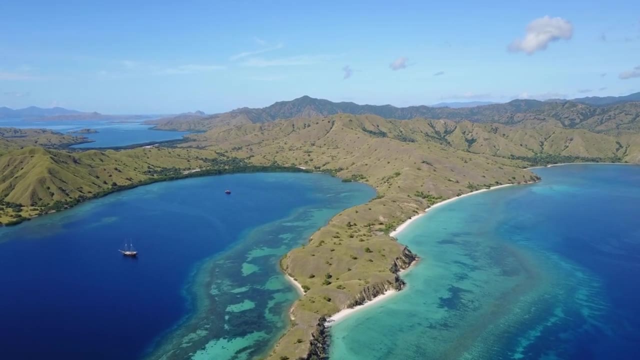 hominin species on the planet during the late Pleistocene. Additionally, the discovery of Homo floresiensis on Flores, an island separated from the Southeast Asian mainland by deep sea channels, raised questions about the species' origins and how it arrived on the island. 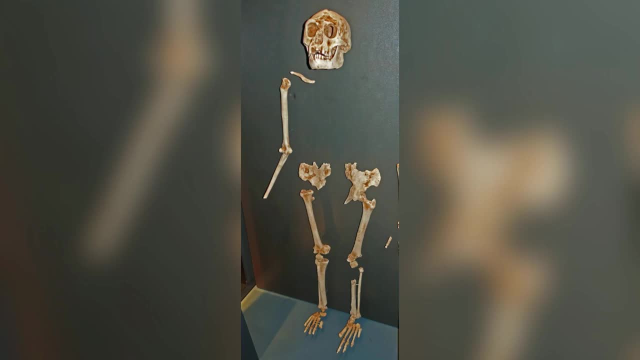 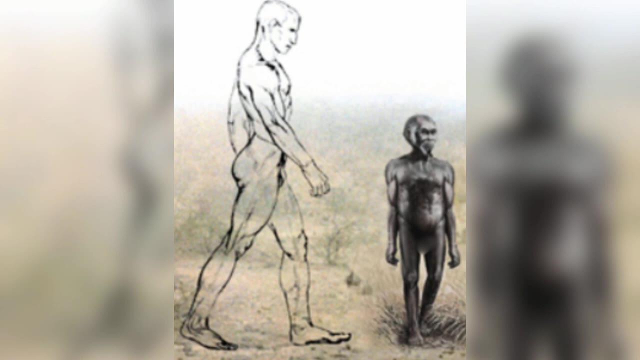 The physical characteristics of Homo floresiensis were equally perplexing. Its small stature and brain size were initially thought to be the result of pathological dwarfism or island dwarfism, a phenomenon where species evolve smaller body sizes when their populations range is limited to a small environment like an island. 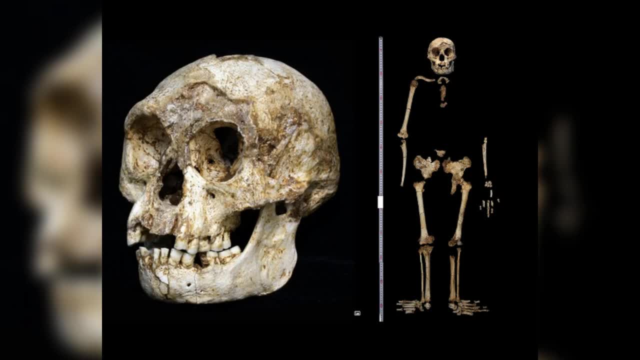 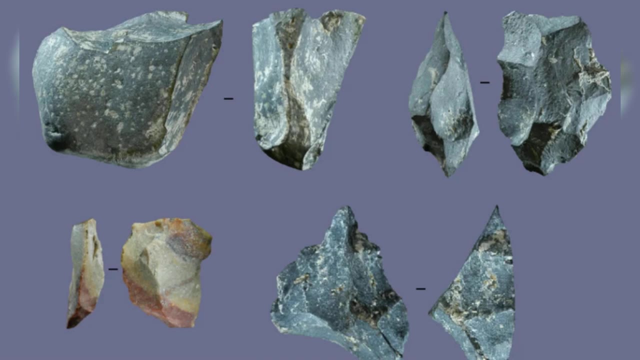 However, further analysis suggested that Homo floresiensis represented a distinct species with unique morphological features that were not merely the result of insular dwarfism. The discovery of stone tools alongside the remains indicated that, despite their small brain size, these individuals were capable tool users, challenging assumptions about the relationship. 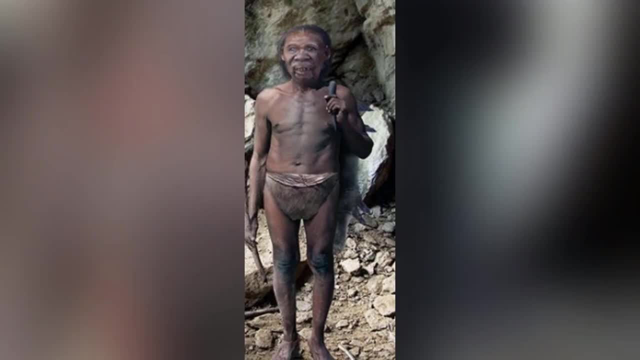 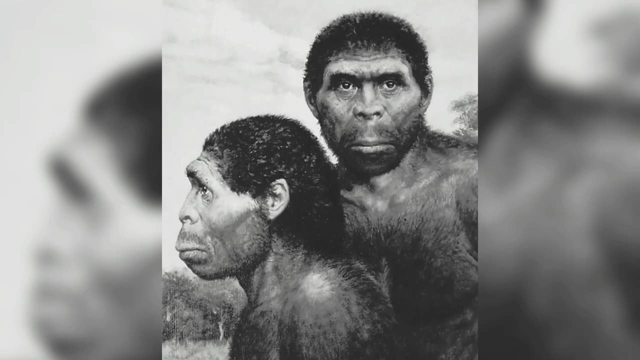 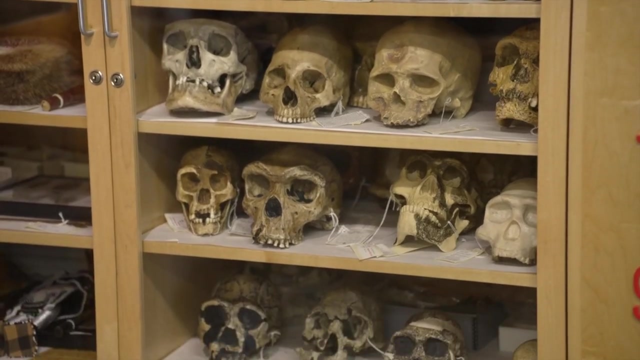 between brain size and cognitive ability. The debate over the origins of Homo floresiensis has been lively. Some scientists propose that it descended from a population of Homo erectus that became isolated on the island and underwent dwarfing. Others suggest it might represent a lineage that branched off earlier in the human family tree. 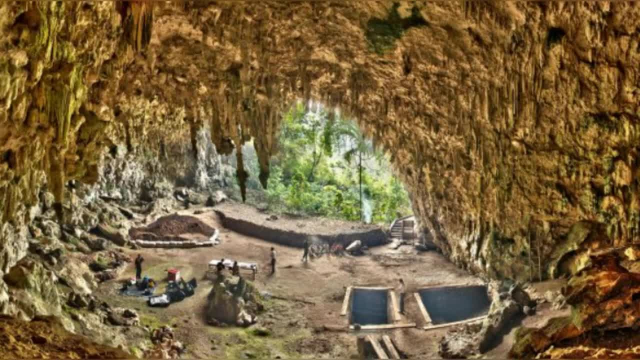 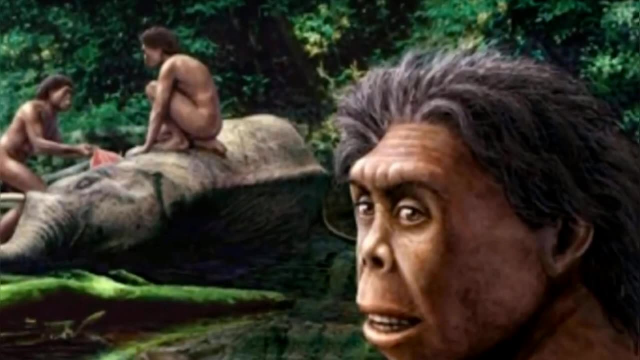 possibly even before the emergence of Homo erectus. The discovery of additional skeletal remains and the ongoing excavation at Liangboa Cave have provided further insights into the life and environment of Homo floresiensis. These include evidence of their diet, the animals they hunted. 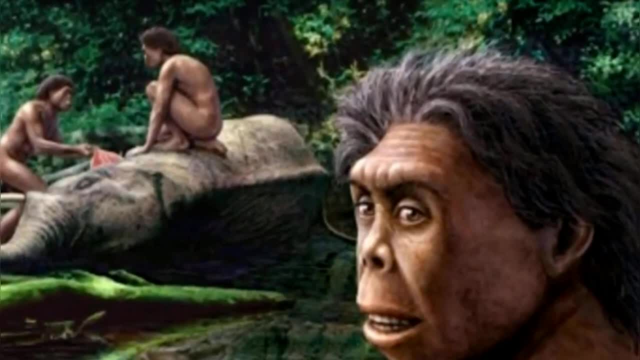 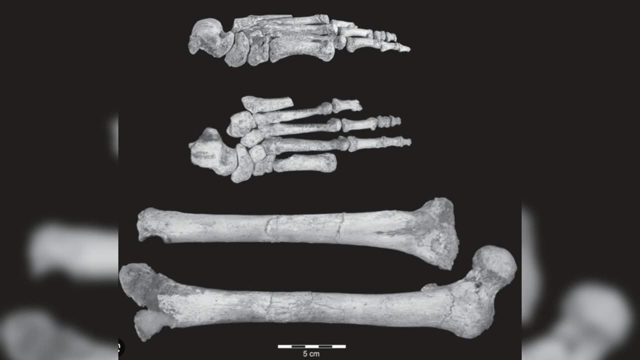 and the potential hazards they faced, such as volcanic eruptions and tsunamis, which may have contributed to their extinction. Homo floresiensis has profoundly impacted our understanding of human evolution, highlighting the incredible diversity and adaptability of hominins. 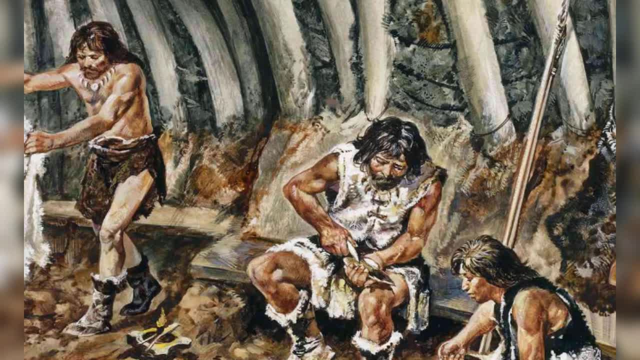 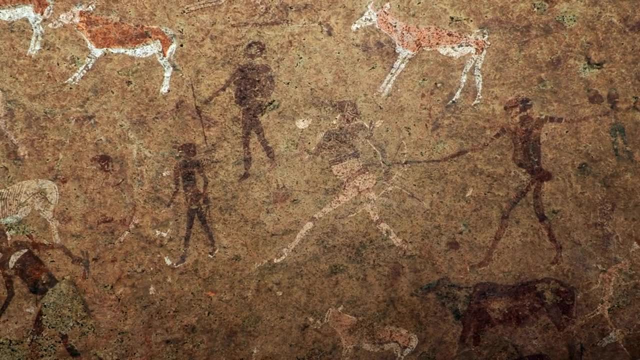 It has opened up new avenues of research into the ways different human species have adapted to their environments and interacted with one another. Their story is a reminder of the mysteries of our past that remain to be discovered and the complexities of the human story that continue. 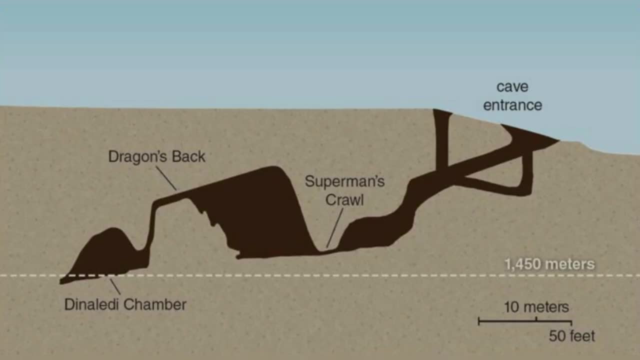 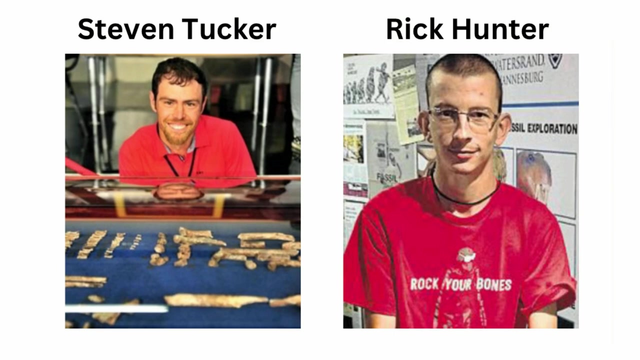 Let's now go to South Africa. The tale of Homo naledi begins with a whisper of curiosity and the lure of the unknown deep within the rising star cave system in the cradle of humankind. South Africa In 2013,. two recreational cavers, Rick Hunter and Stephen Tucker. 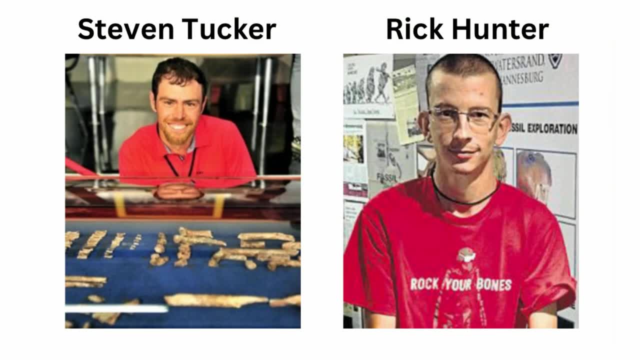 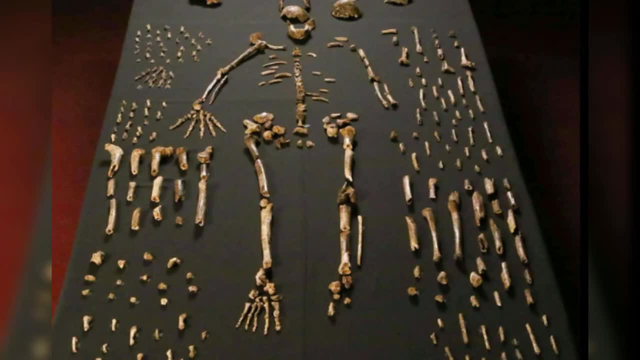 stumbled upon a narrow vertical chute. Squeezing through this chute, they descended into a chamber that few had ever seen. What they found there was extraordinary: A cache of bones, eyes and bones- Bones untouched and unseen for millennia, scattered across the cave floor. 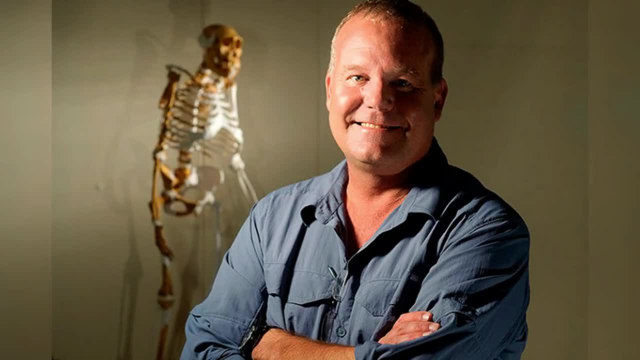 This discovery prompted paleoanthropologist Lee Berger of the University of the Witwatersrand to assemble a team of scientists and specialized cavers for an unprecedented excavation- The team known as the Underground Astronauts. due to the challenging conditions of the cave. 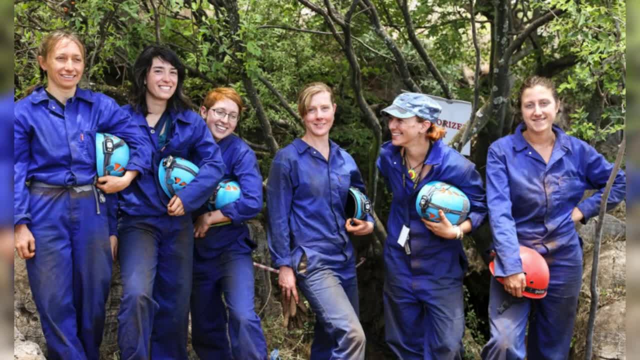 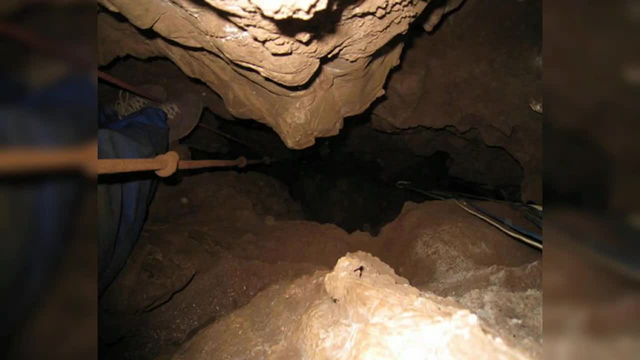 included six women selected for their scientific expertise and ability to navigate the cave's narrow passages. What they unearthed in the cave in the weeks that followed was nothing short of revolutionary. The chamber was filled with the remains of a previously unknown species of hominin. 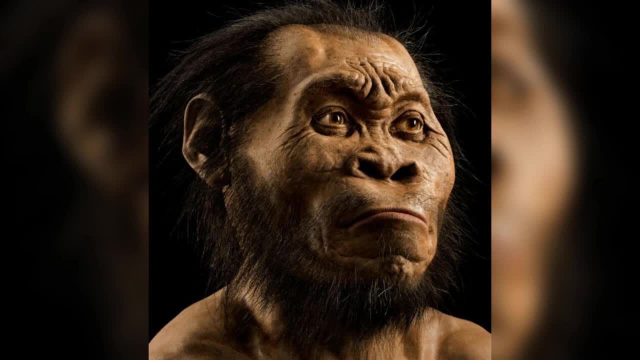 which Berger and his team named Homo naledi, where naledi means star in Sesotho, a local South African language, reflecting the cave's name. Rising Star Homo naledi is enigmatic because of its mosaic of features. 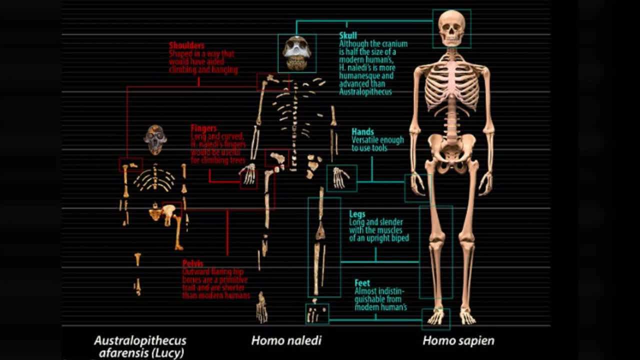 The species exhibited a surprising blend of primitive traits akin to our earliest ancestors, such as a small brain and curved fingers for climbing, alongside more advanced characteristics such as legs and feet, fashion for walking upright. a hallmark of humanity, The hands of Homo naledi with their precise ability to manipulate objects. 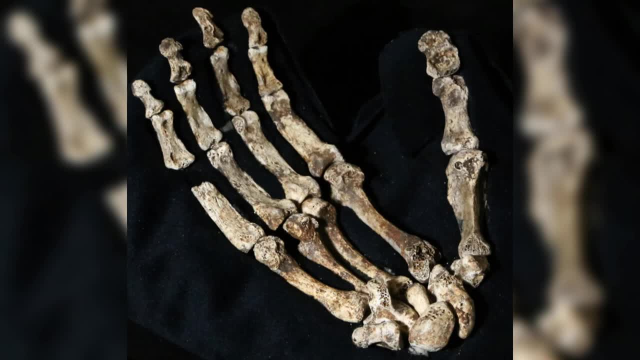 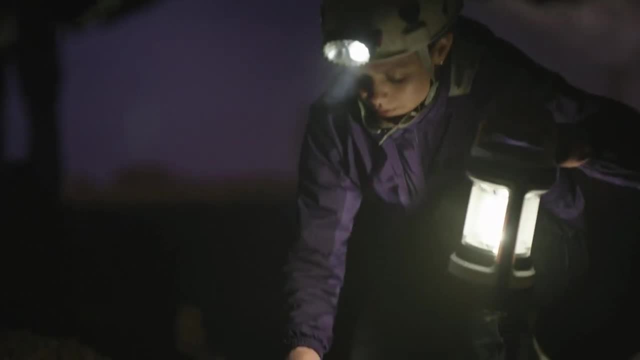 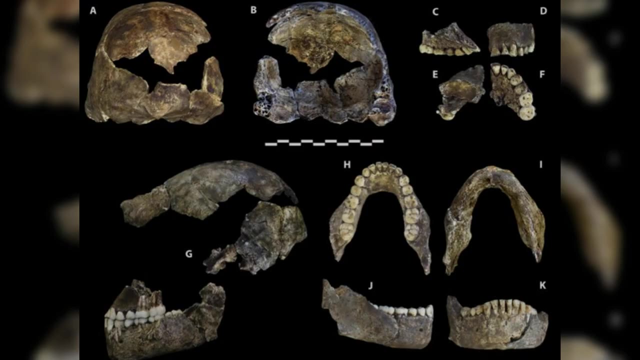 suggest a species that was not only adept at moving through complex terrains, but also capable of using tools. Initially dating the remains proved challenging due to the difficult nature of the cave environment and the absence of typical dating materials. However, subsequent research published in 2017 revealed that the Homo naledi fossils 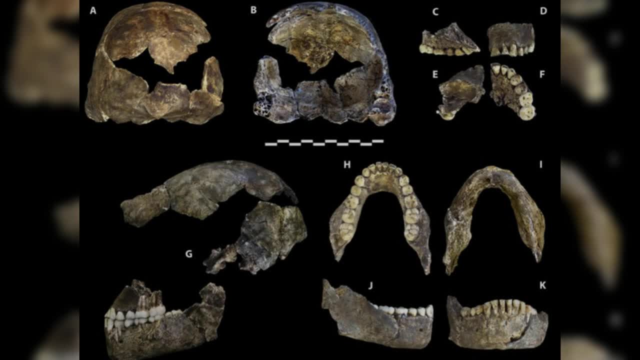 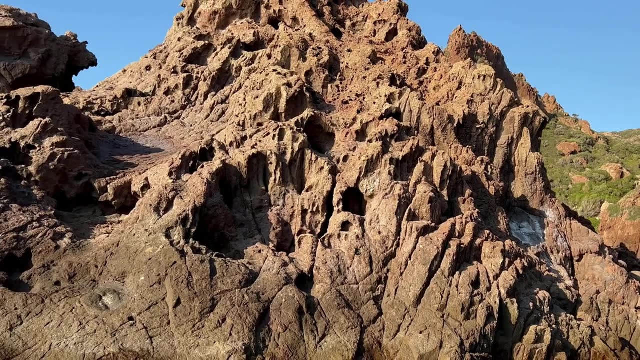 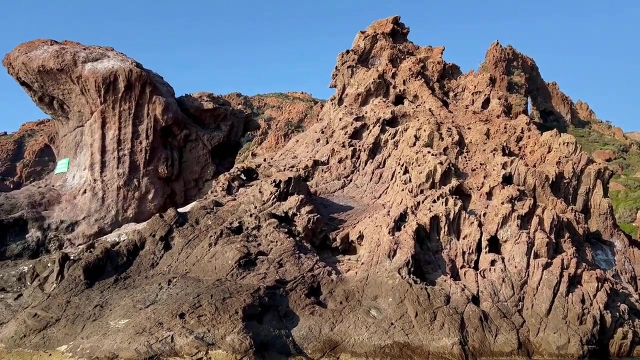 were surprisingly young, dating to approximately 236,000 to 335,000 years ago. This dating places Homo naledi in the late Middle Pleistocene, a period when it was previously thought that only Homo sapiens roamed Africa. The implications of this finding are profound, suggesting a much more complex narrative of 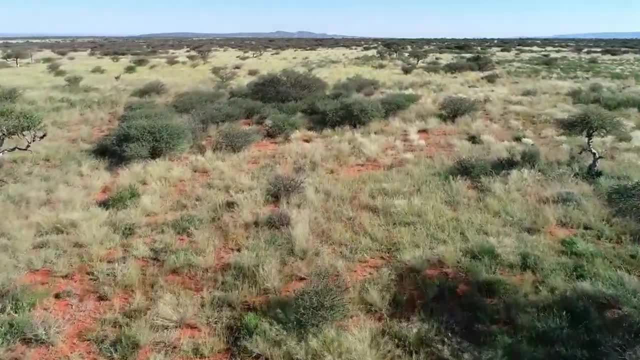 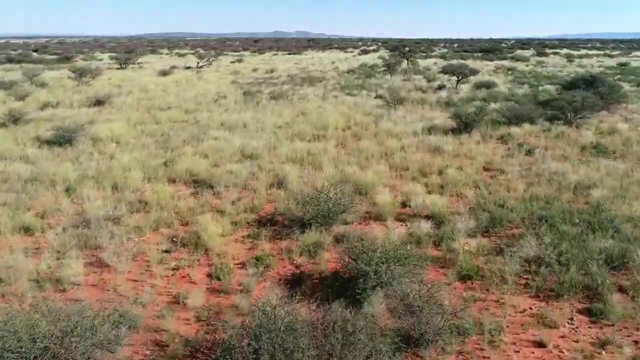 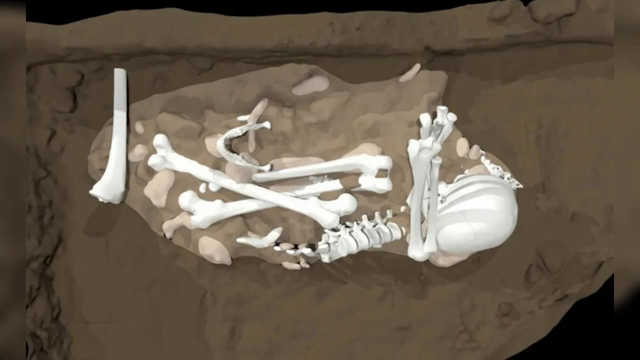 human and animal species. Homo naledi is also known as Homo sapiens. The Homo sapiens are the most common species of human evolution than previously understood, with multiple species of hominins potentially coexisting on the African continent. Perhaps the most mystifying aspect of the Homo naledi discovery is the context in which 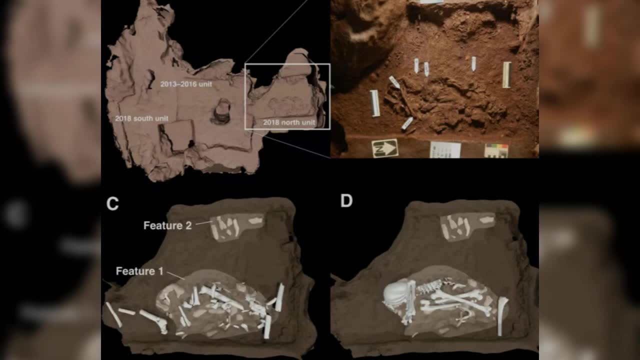 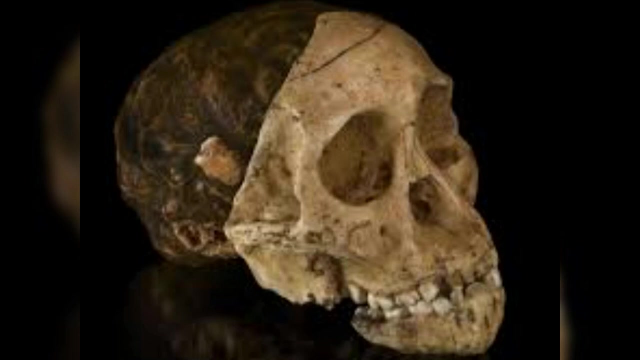 the remains were found. The deliberate placement of bodies in the remote chamber of the cave hints at a rudimentary form of ritual behavior or an understanding of death, traits previously attributed exclusively to species with much larger brains In Africa in 1924, the discovery of the Taong child marked a pivotal moment in the field. 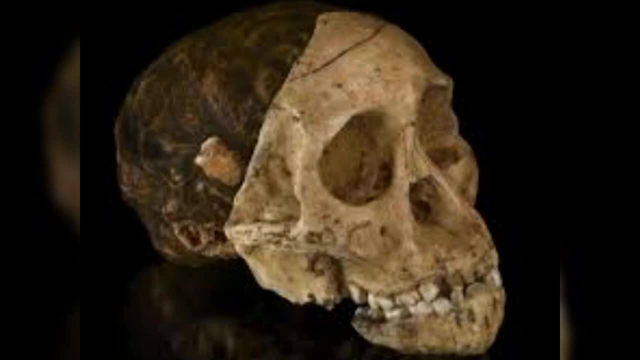 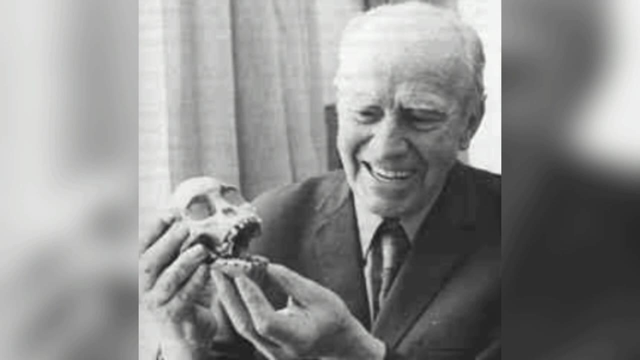 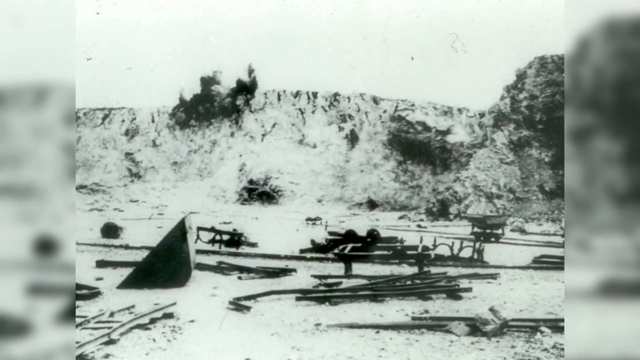 of paleoanthropology and forever altered our understanding of human evolution. Raymond Dart, an Australian anatomist and anthropologist working at the University of Witwatersrand in Johannesburg, South Africa, was the scientist behind this groundbreaking find. The story began when Dart received a box of fossil-bearing rocks sent by workers at 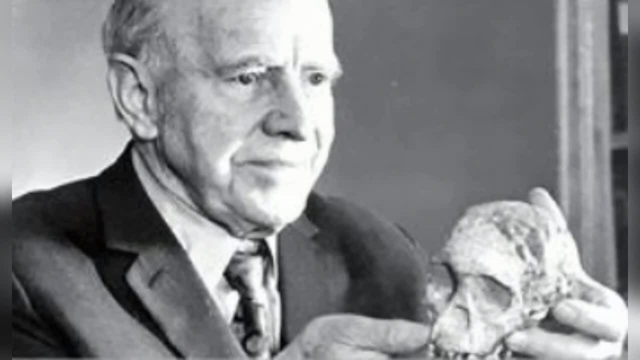 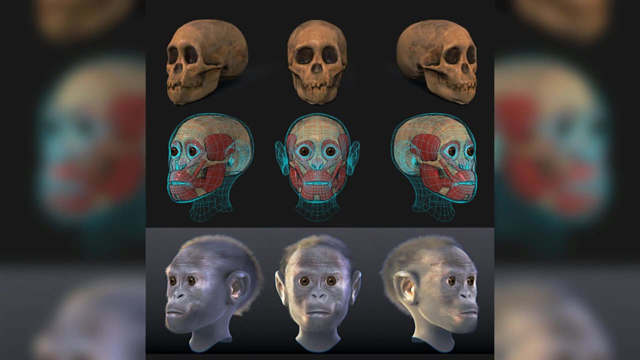 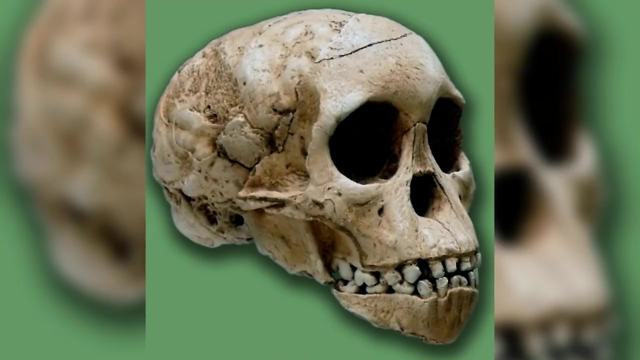 a limestone quarry in Taong, South Africa. Among these rocks, Dart noticed a small fossilized skull that appeared to be that of a young ape. However, upon closer examination, Dart realized that he had stumbled upon something far more significant. The skull, belonging to a juvenile individual, exhibited a unique combination of features. 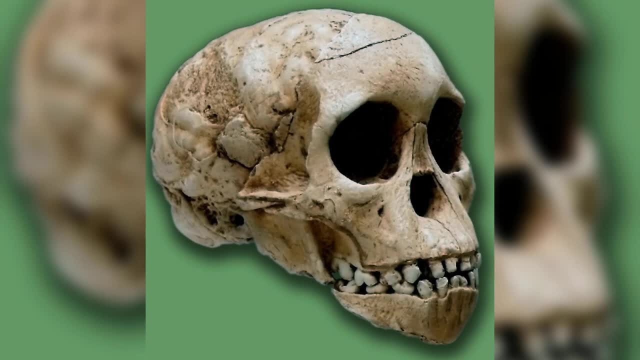 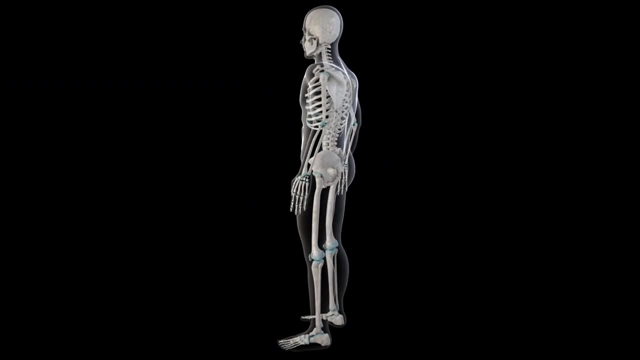 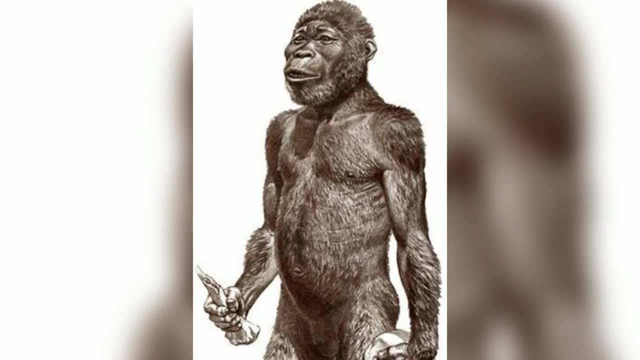 long, long, long, long long, But it wasn't long enough to see that this individual walked upright- a key characteristic of hominins. the group that includes humans. Dart identified the specimen as a new species, which he named Australopithecus africanus. 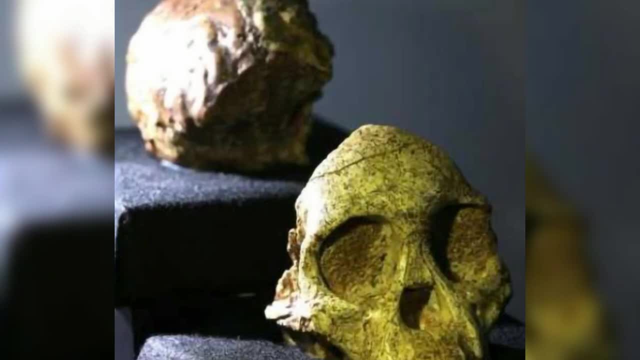 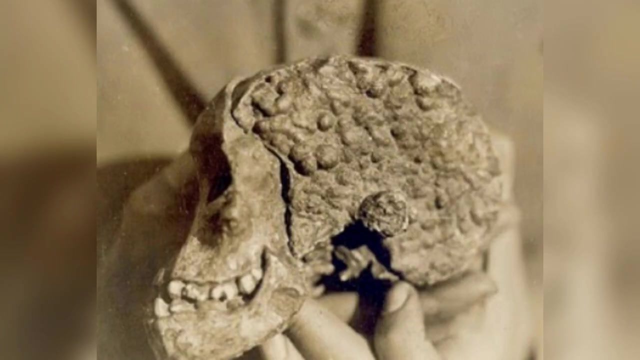 meaning Southern Ape of Africa. He proposed that this small-brained, upright walking creature was an early human ancestor, challenging the prevailing view that early hominins would be found in Europe or Asia and would have large brains similar to modern humans. The publication of Dart's findings in 1925. 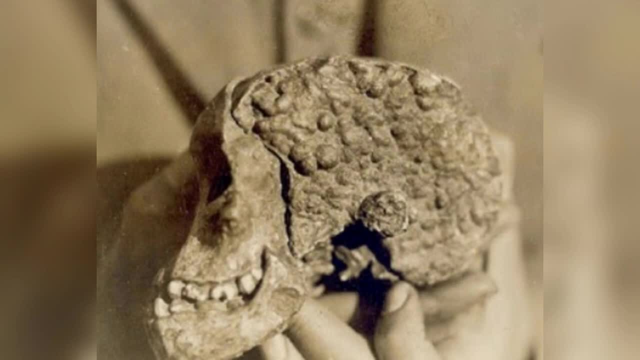 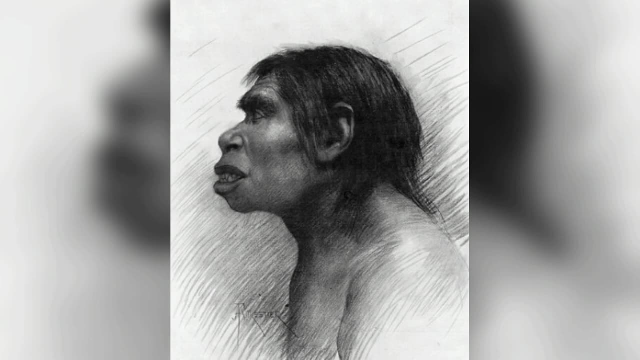 was met with scepticism by many in the scientific community. At the time, the dominant theory of human evolution centred around the Piltdown Man, a fossil find in England that was later revealed to be a hoax. Many scientists were reluctant to accept the idea. 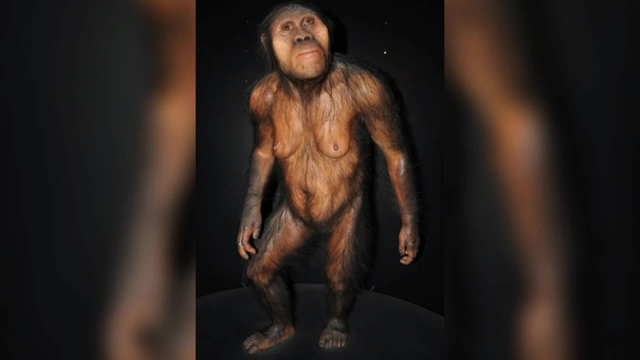 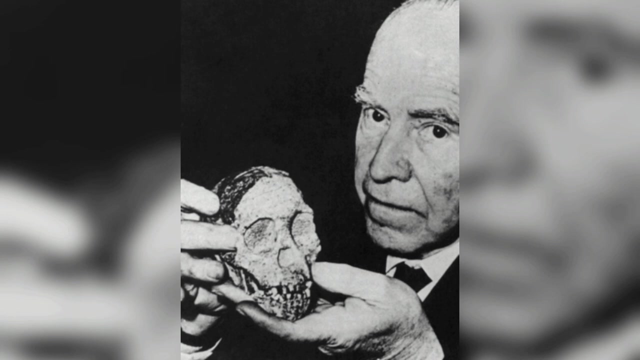 that the cradle of humankind might be in Africa, and Dart's Australopithecus africanus did not fit their expectations of what an early human ancestor should look like. Despite the initial controversy, the Taung child gradually gained recognition as a crucial piece of the human evolution puzzle. 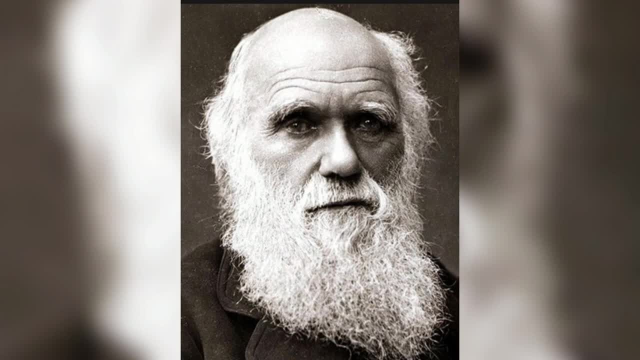 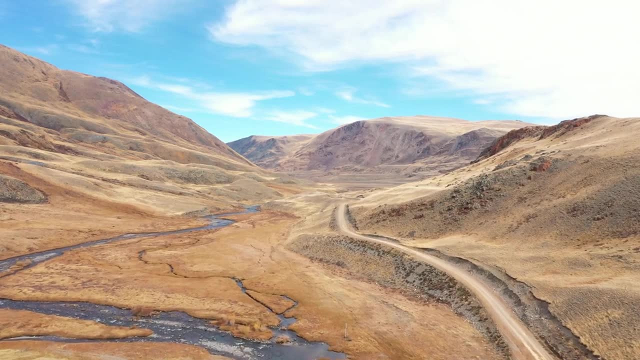 The discovery provided the first evidence of an early hominin species in Africa, supporting Charles Darwin's earlier speculation that humans originated on this continent. Over the years, further discoveries of Australopithecus species in Africa reinforced Dart's findings and shifted the focus of paleontologists. 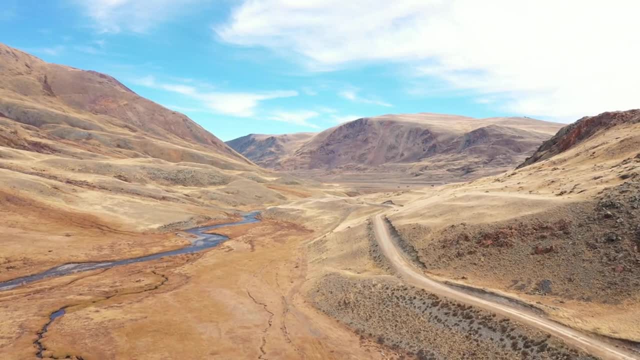 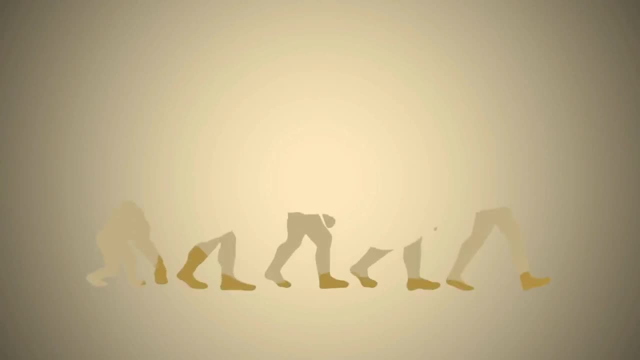 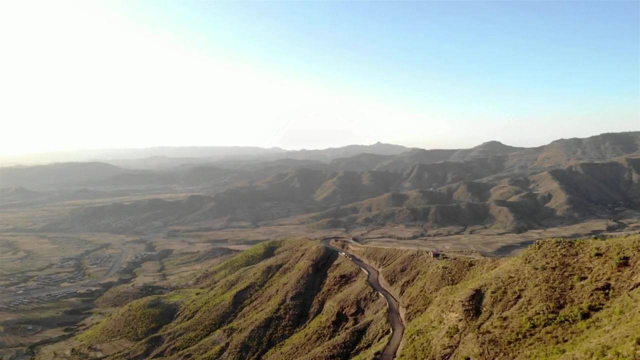 paleoanthropological research to the African continent, where the richest evidence of human evolution has since been found. The Taung child remains one of the most famous and important fossil discoveries in the study of human evolution. Let's go back to Afar region of Ethiopia once more. 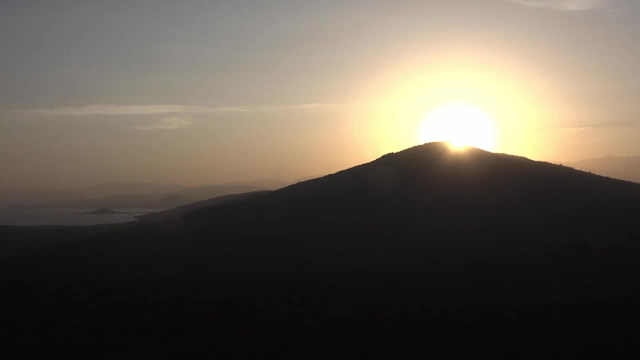 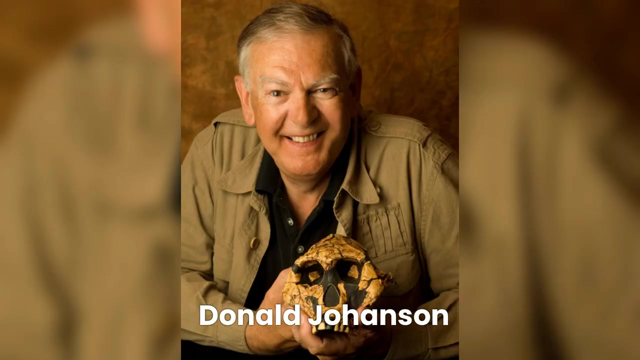 In November 1974, a monumental discovery was made in the remote reaches of the Afar region of Ethiopia. A young paleoanthropologist named Donald Johansen, alongside his graduate student, Tom Gray, embarked on what would become one of the most significant expeditions. 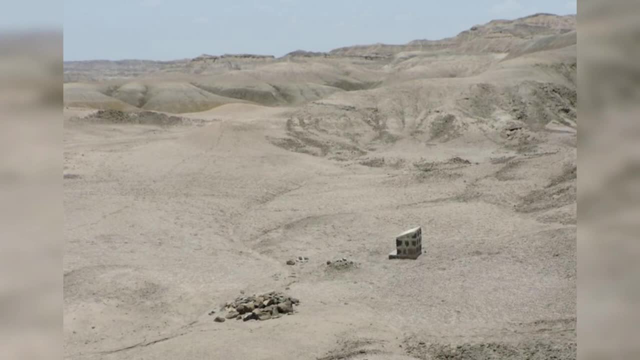 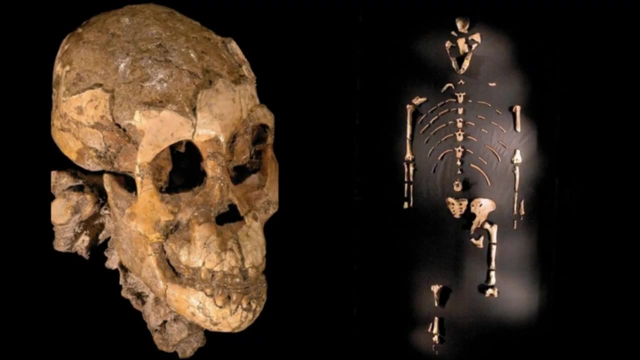 in the study of early humans. As they navigated the harsh landscape near the village of Hadar, their attention was caught by a fragment of an elbow bone protruding from the barren ground. This seemingly modest find led them to uncover the remains of a female hominin who lived 3.2 million years ago. She would come to be known affectionately as Lucy, named after the Beatles' song Lucy in the Sky with Diamonds, which played in the expedition camp that jubilant evening. Lucy's skeletal remains, catalogued as AL2881,, represented a new species: Australopithecus afarensis. 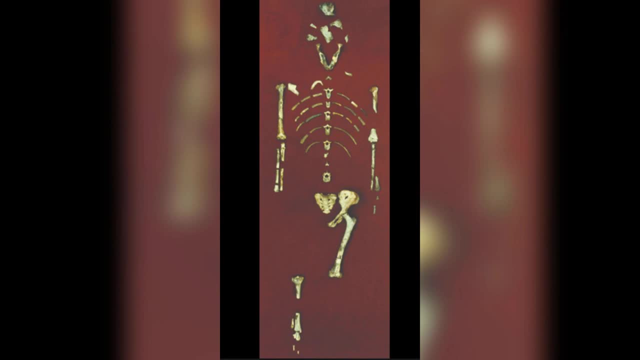 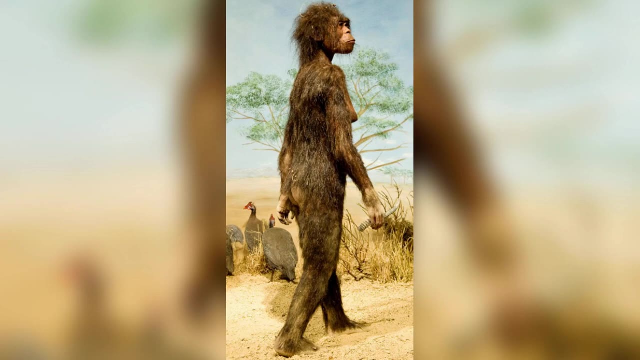 With 40% of her skeleton recovered. Lucy provided an unprecedented glimpse into the life of early hominins. She had a small stature, standing at about 3.5 feet tall, and her cranial capacity was similar to that of a chimpanzee. 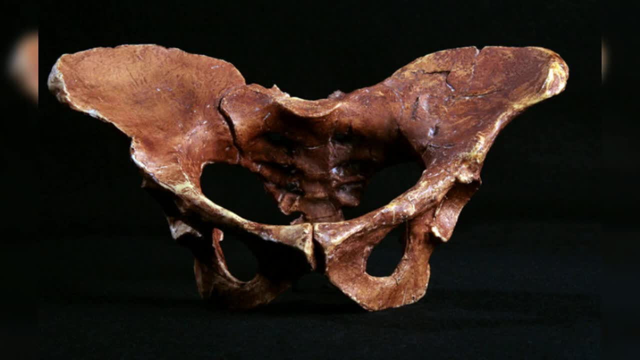 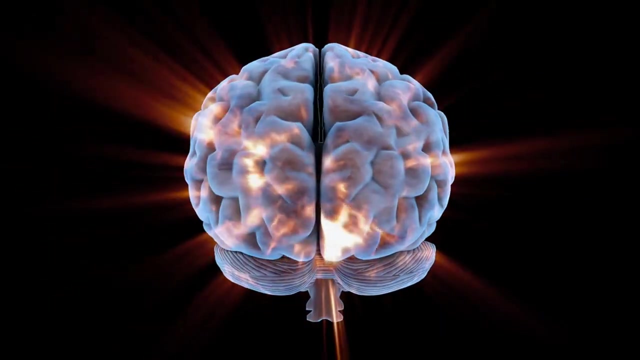 However, it was her pelvic structure, knee and leg bones that offered groundbreaking evidence of bipedal locomotion, suggesting that Lucy and her kin walked upright on two legs. The discovery of Lucy challenged the prevailing theory of the time, which posited that brain size increased before bipedalism. 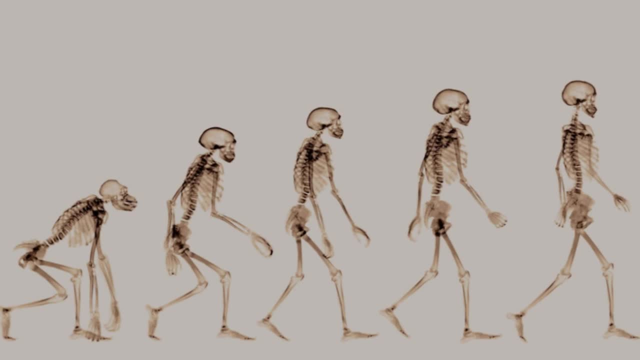 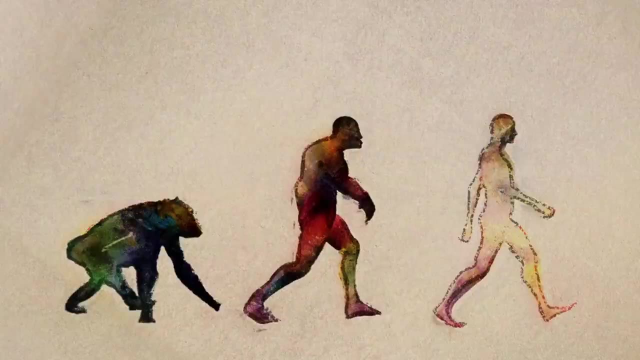 Lucy's existence proved that bipedalism predated significant brain enlargement. This finding had profound implications for the scientific community's understanding of the adaptive strategies that shaped human evolution, emphasizing the importance of bipedalism in early human development. The site where Lucy was discovered, the Hadar Formation- 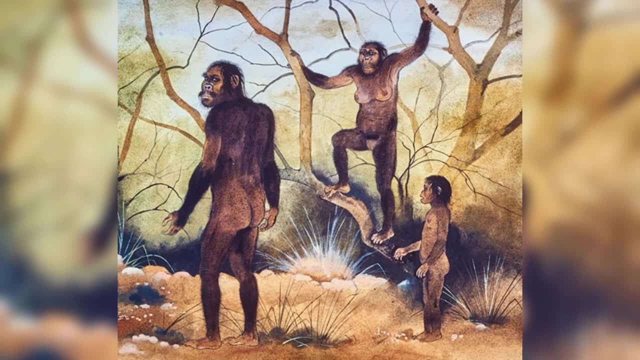 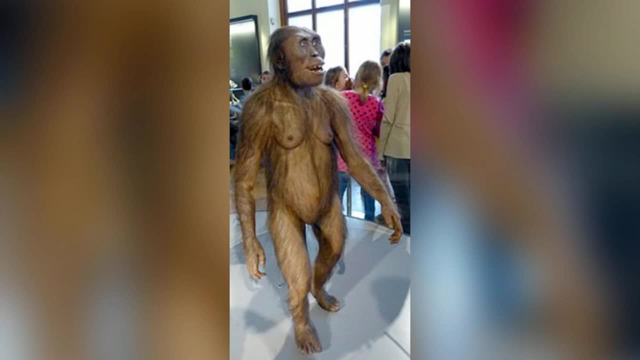 has since yielded additional fossils of Australopithecus afarensis, providing further insights into the species' morphology and lifestyle. Over the years, Lucy has captivated the imagination of both scientists and the public alike, becoming an icon of human evolutionary research. 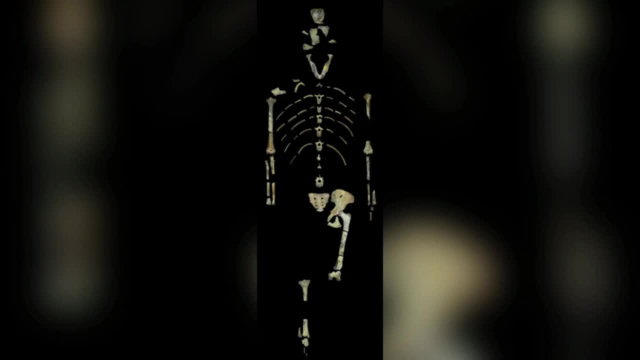 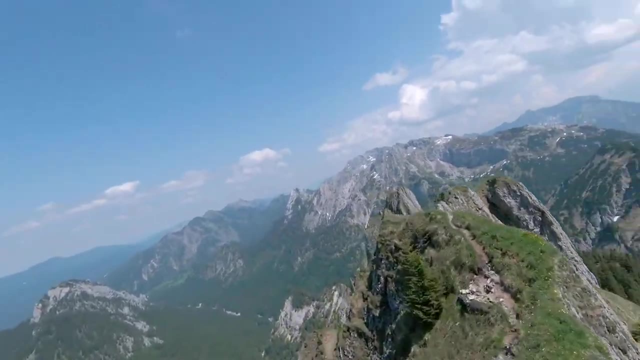 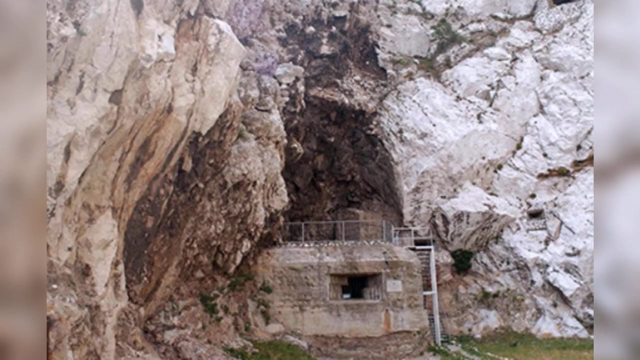 Her remains are among the most studied and celebrated of all hominin fossils, serving as a tangible connection to our distant ancestors. Let's go to Germany now to meet our closest extinct relative. The story of the discovery of Neanderthals begins in the summer of 1856 in the Neander Valley. 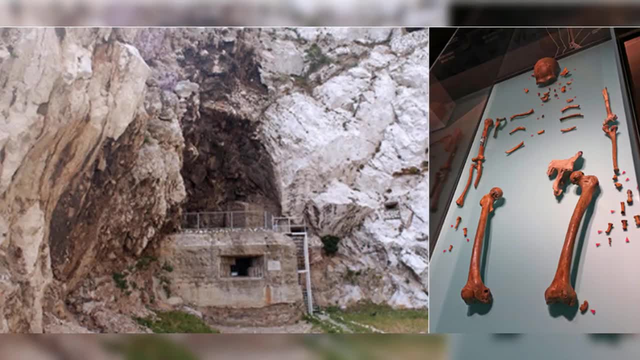 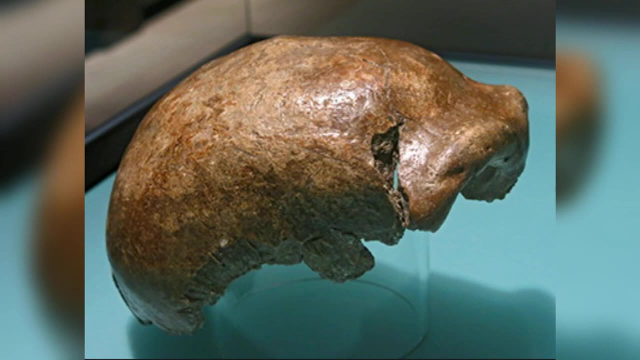 near Düsseldorf, Germany, Quarry workers stumbled upon a set of unusual bones within a limestone cave, not realizing they had just found the first recognized fossils of our closest extinct human relatives, the Neanderthals. Neanderthals: These fossils included parts of a skull, some limb bones and ribs. The bones were 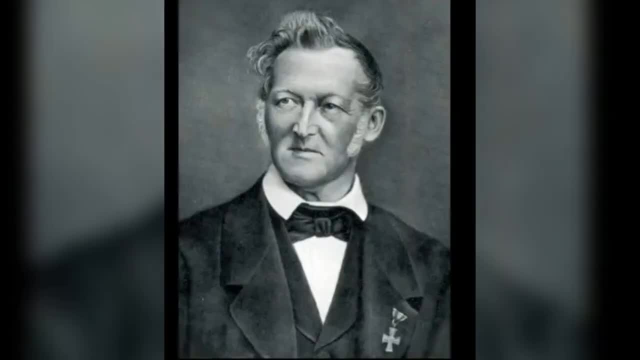 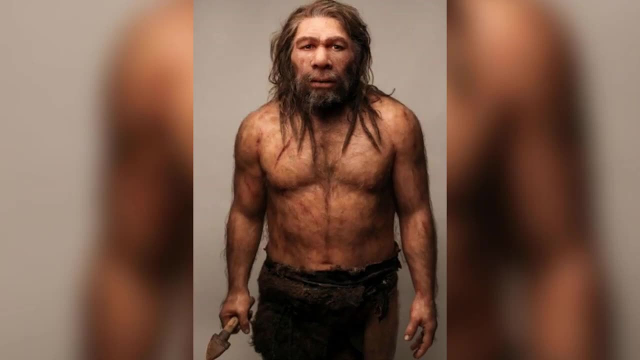 given to a local schoolteacher and amateur naturalist, Johann Karl Fuhlroth, who immediately recognized their significance. Fuhlroth, in collaboration with anatomist Hermann Scharfhausen, presented the findings to the scientific community, suggesting that these bones belonged. 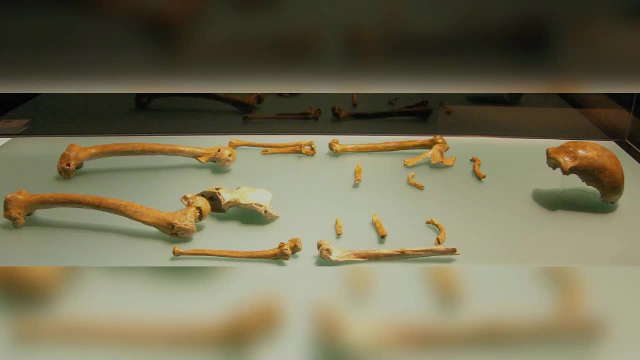 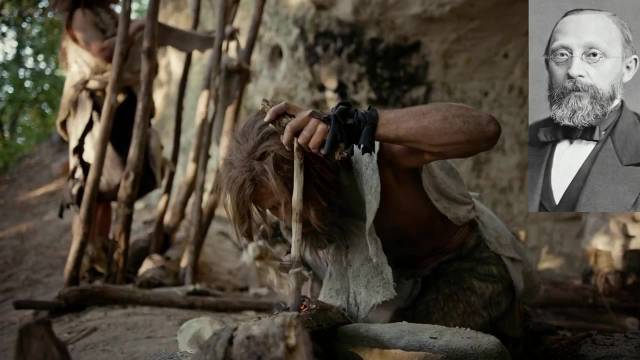 to an ancient human form. The discovery of the Neanderthal remains sparked considerable debate among scientists of the time. Some saw these fossils as evidence of a distinct human species that had once lived in Europe, while others, including prominent figures such as Rudolf Virchow. 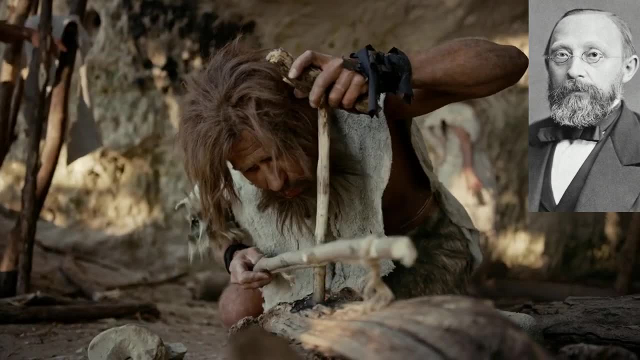 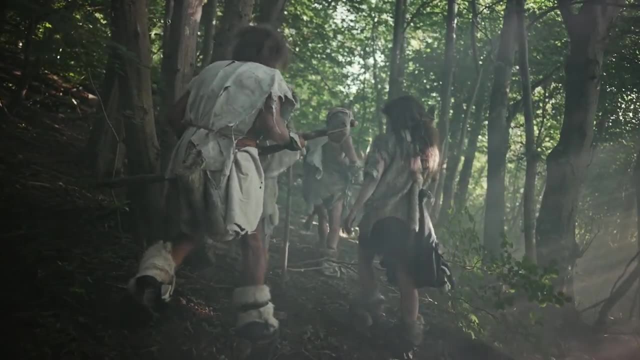 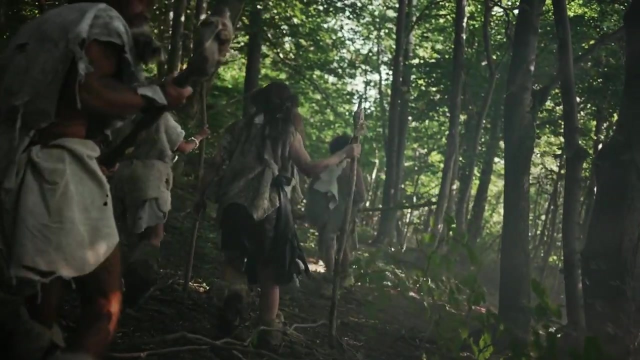 dismissed them as the remains of a modern human afflicted with disease. This skepticism was rooted in the prevailing beliefs about human uniqueness and the lack of a comprehensive framework for understanding human evolution, a framework that Charles Darwin would provide just a few years later, with the publication of 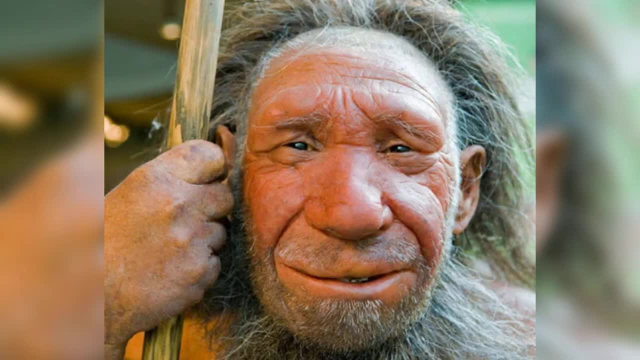 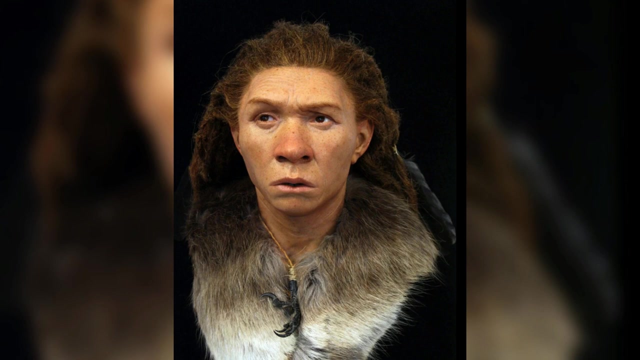 On the Neanderthal On the origin of species. The initial Neanderthal fossils were characterized by a robust skeleton with a large, low-sloping skull, a pronounced brow ridge and a lack of a prominent chin. These features were markedly different from those of modern humans, challenging the then-existing views on human variability. 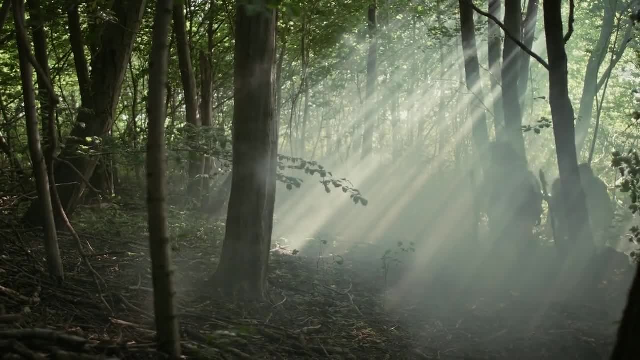 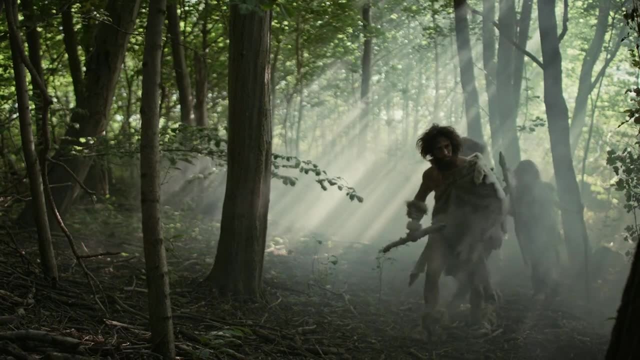 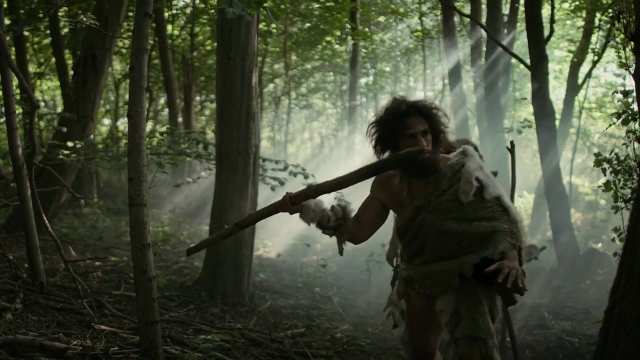 and evolution. Despite early resistance, the distinctiveness of Neanderthal anatomy eventually became undeniable, especially as more Neanderthal fossils were discovered. Neanderthals were discovered across Europe and parts of Asia, showing consistent patterns of morphology that differed from those of modern humans. The Neander Valley discovery and subsequent 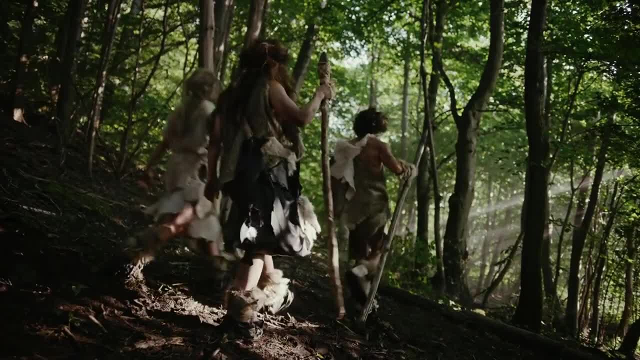 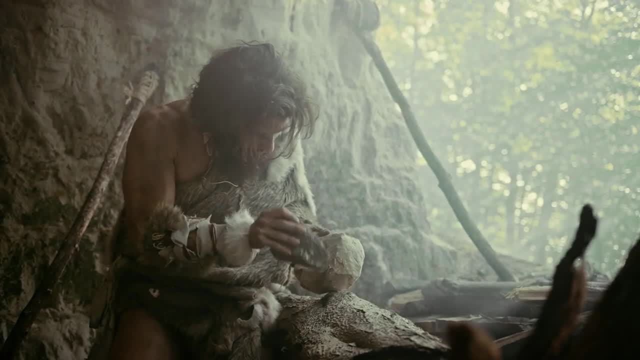 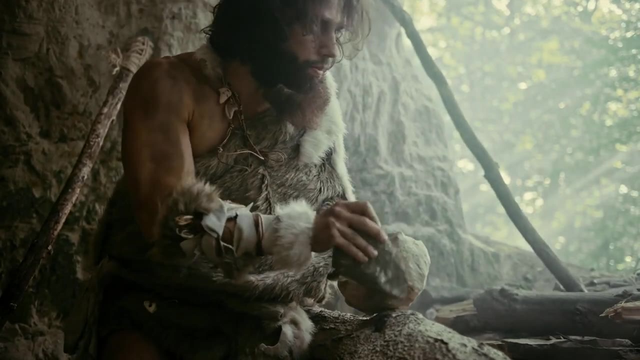 finds painted a picture of a widespread group of hominins that had adapted to the harsh conditions of Ice Age Europe. Neanderthals were skilled toolmakers and hunters, with evidence suggesting they had complex social structures and may have practiced burial rituals for their dead. 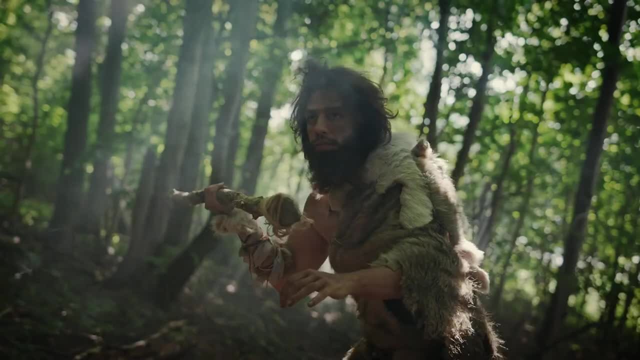 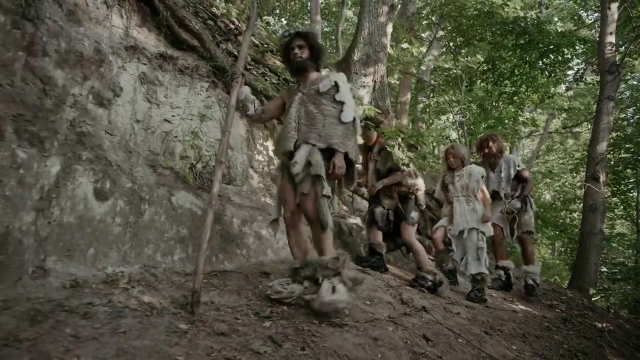 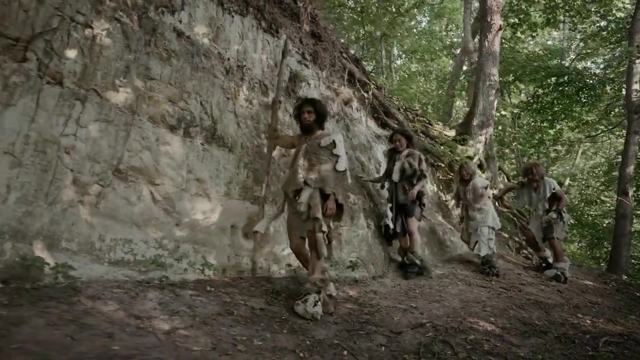 indicating a capacity for symbolic thought. The significance of Neanderthals in our understanding of human evolution cannot be overstated. They represent a parallel lineage that lived alongside and at times interbred with our own ancestors, contributing to the genetic makeup of modern humans outside. 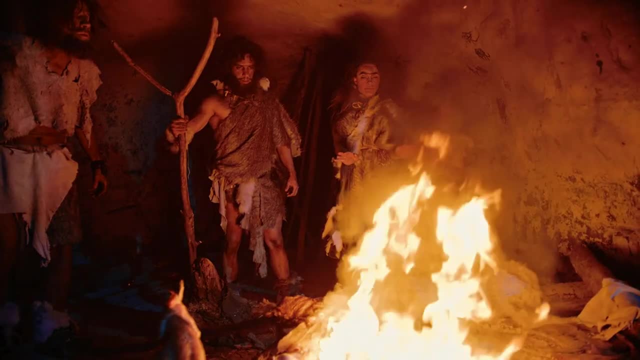 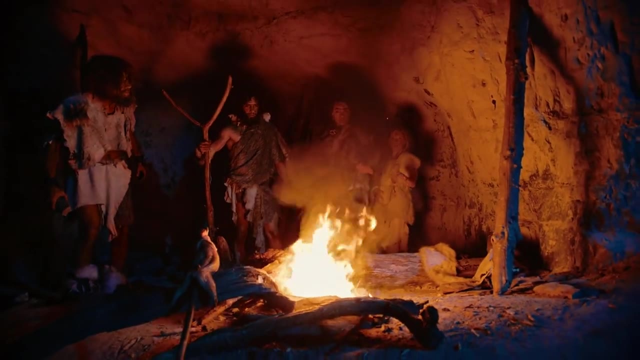 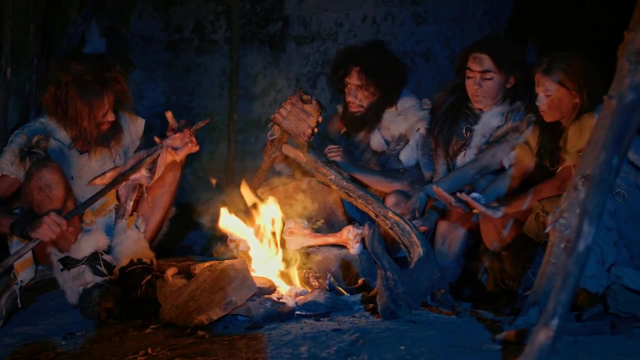 Africa. The discovery of Neanderthals challenged Victorian assumptions about the linear progression of human evolution and the uniqueness of human beings, highlighting the complexity and depth of our shared ancestors. Today, Neanderthals are recognized as a crucial part of the human story, offering invaluable 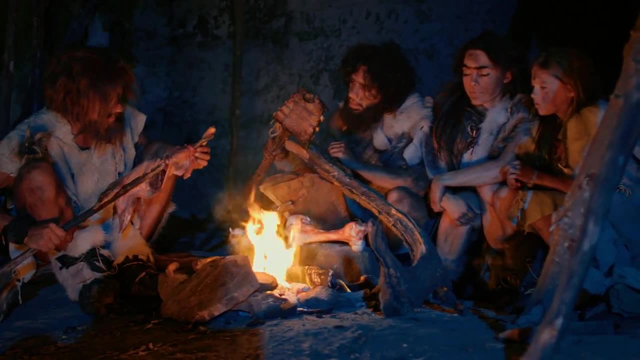 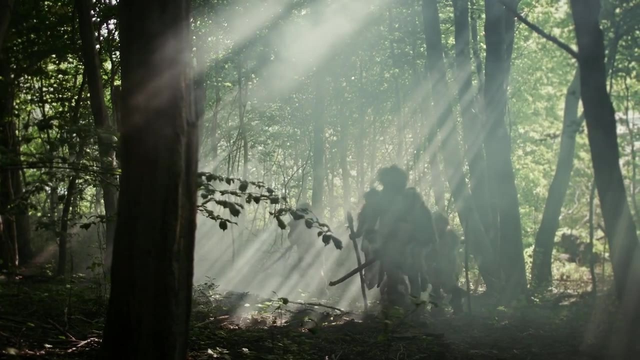 insights into our evolutionary past, our capacity for adaptation and the shared characteristics that define what it means to be human. The discovery in the Neander Valley laid the groundwork for paleoanthropology as a scientific discipline and opened the door to further discoveries. 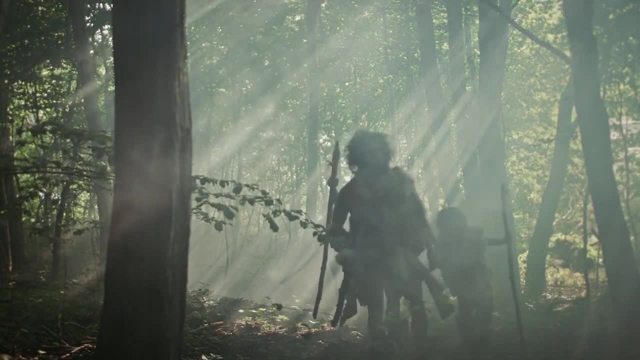 that continue to enrich our understanding of human history. Thanks for watching. Please like and subscribe for more such videos. Thanks for watching. Please like and subscribe for more such videos. Thanks for watching. Please like and subscribe for more such videos.